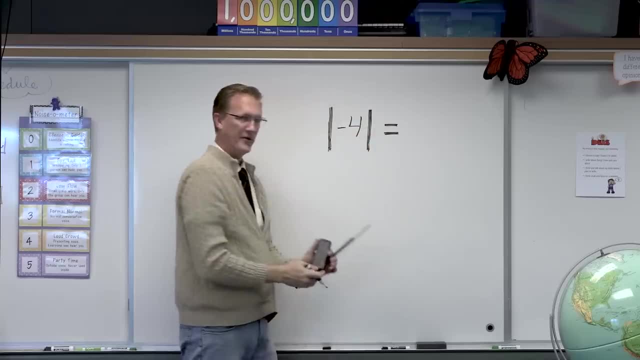 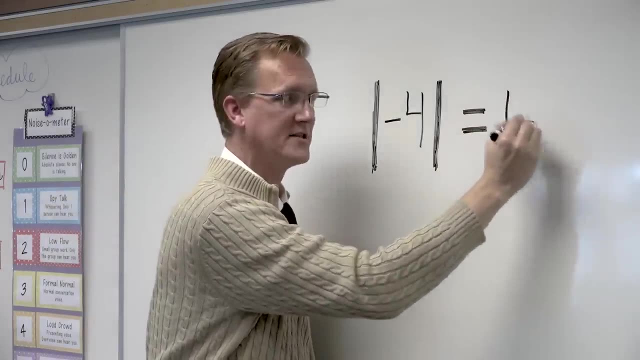 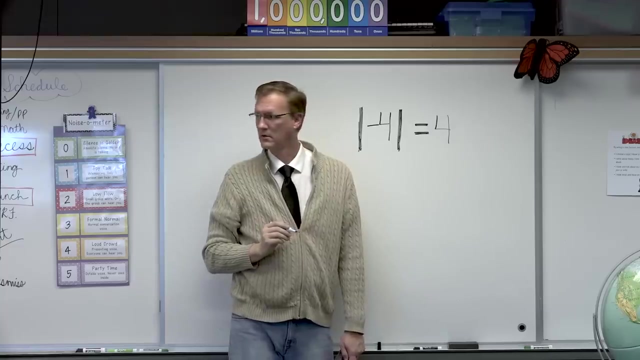 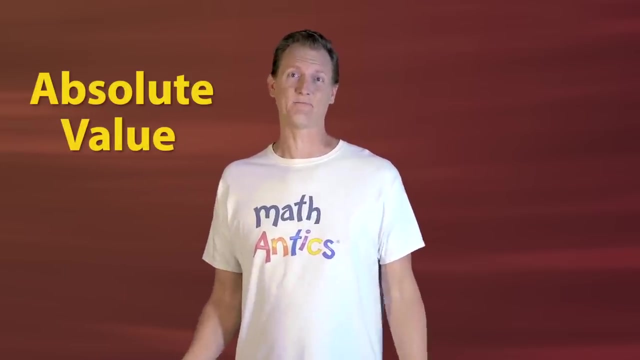 then, just like magic, it comes out positive. Any questions? Well, maybe it wasn't quite that bad, But absolute value sure seemed a lot less exciting than the name suggested. It seemed like just a way to turn a negative number into a positive one. 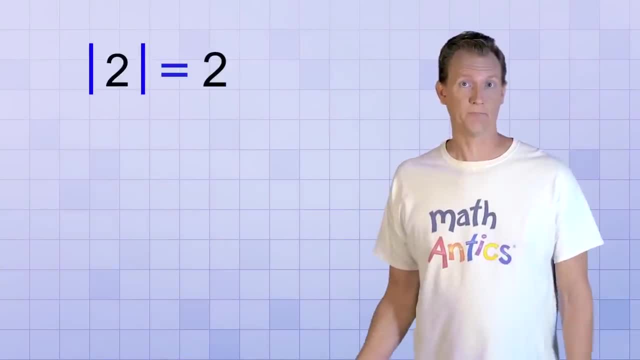 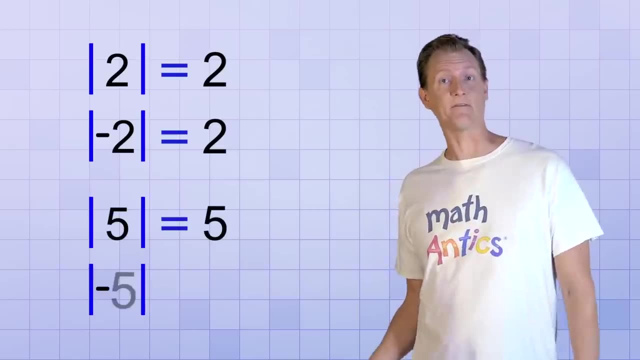 For example, the absolute value of 2 is 2, but the absolute value of negative 2 is also 2.. The absolute value of 5 is 5,, but the absolute value of negative 5 is also 5.. See those vertical lines on either side of the numbers. 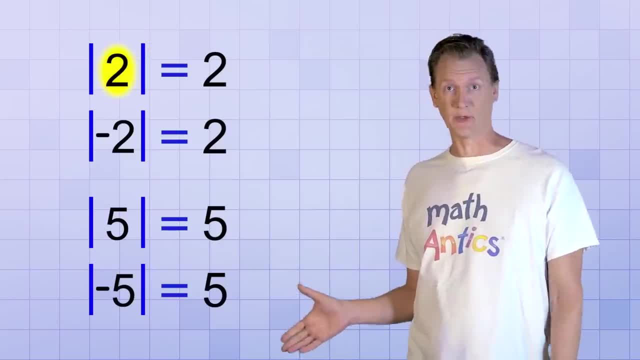 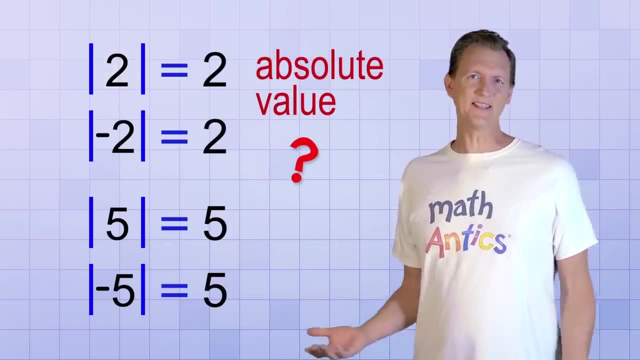 That's the symbol used for absolute value. So when you see something in between those vertical lines, it means to find the absolute value of it. But what does absolute value even mean? From these examples, it seems like it's just the positive version of any number. 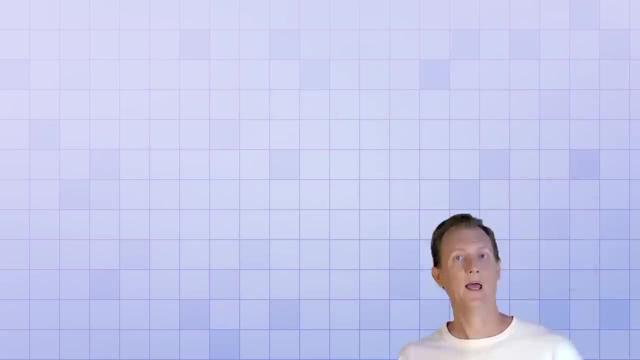 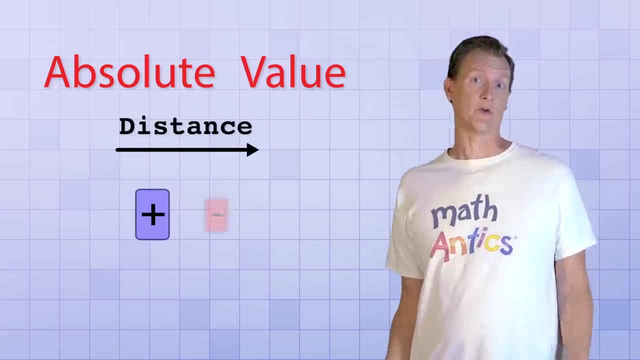 Well, sort of, but it's a little more involved than that. Absolute value is a more general concept in math that actually has more to do with the idea of distance than it does with the idea of positive or negative numbers. It's usually introduced in basic math right after you learn about negative numbers. 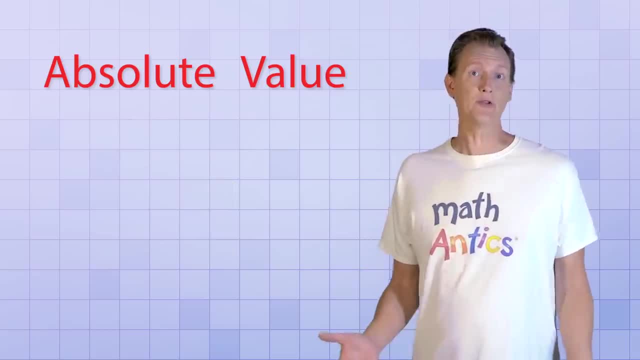 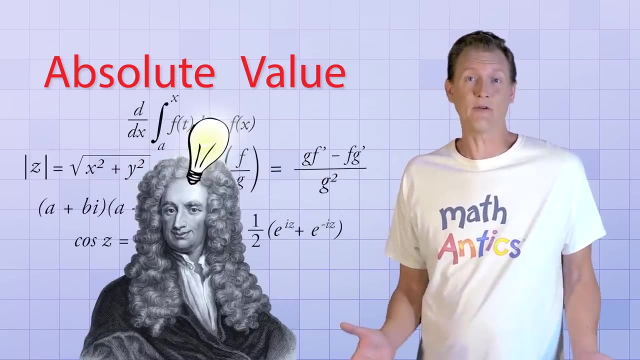 But absolute value is a concept that's even more useful and more interesting in advanced math. Because of that, I'm going to teach you about absolute value using an idea that you usually don't encounter until a little later on in your math journey, And that idea is vectors. 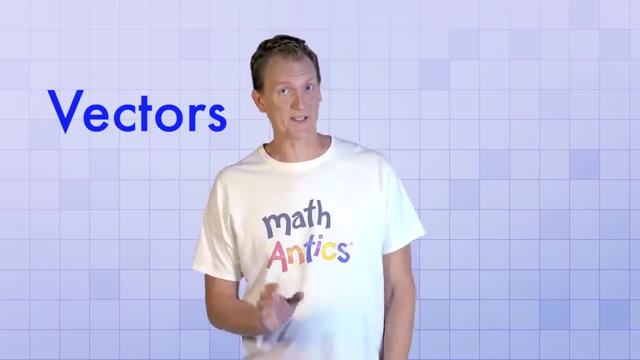 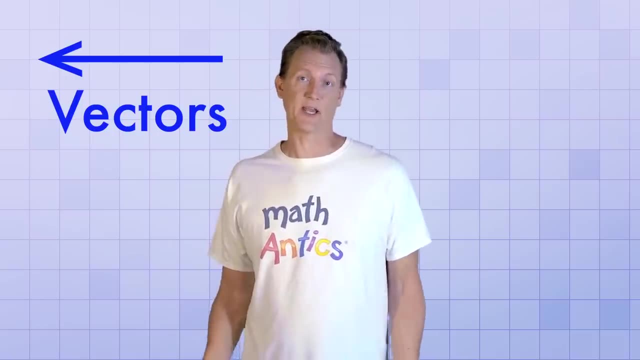 The term vector might sound kind of technical, but they're actually really simple. Vectors are basically just arrows. In real life, an arrow can have all sorts of different properties. For example, this arrow is made of wood and has feathers, while this arrow is red plastic with a round thingy at the end. 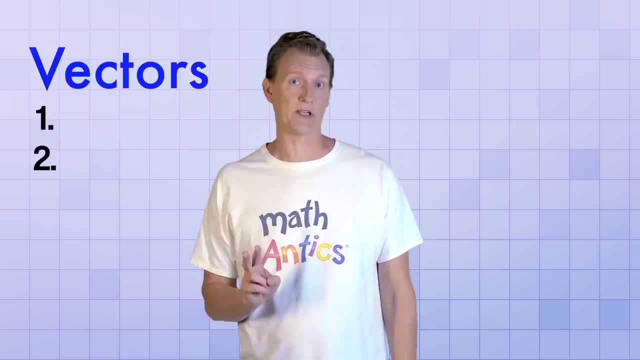 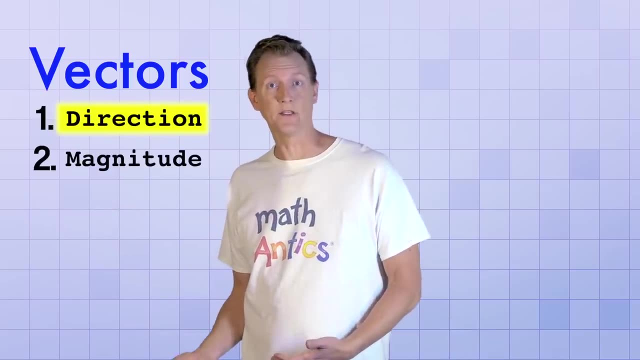 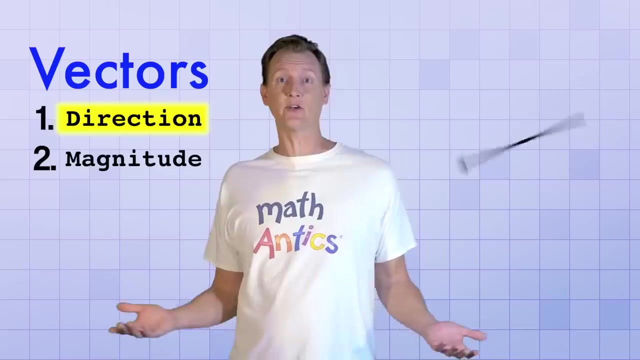 But in math the arrows we call vectors only have two properties: They have a direction and a magnitude. What do those two properties mean? That is pretty obvious. It's just which way the arrow or vector is pointing. It could be up down, left, right or just about any direction you can think of. 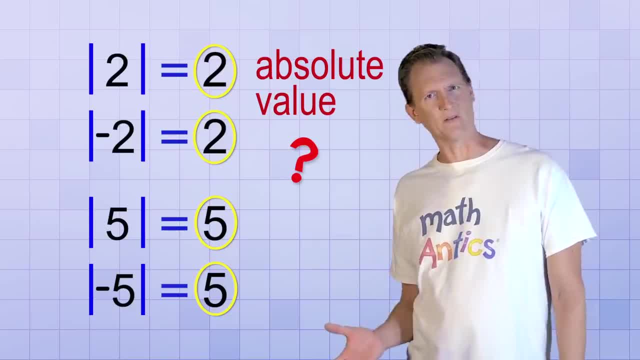 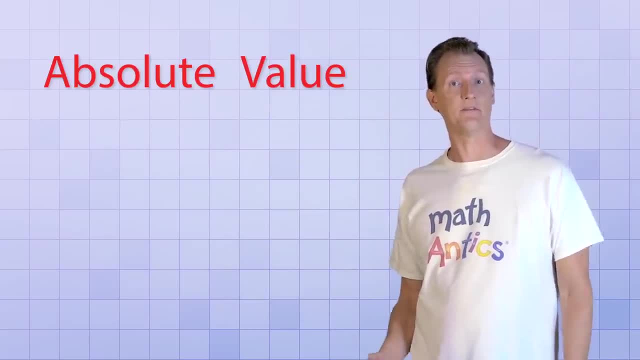 the positive version of any number, Well sort of, but it's a little more involved than that. Absolute value is a more general concept in math that actually has more to do with the idea of distance than it does with the idea of positive or negative numbers. 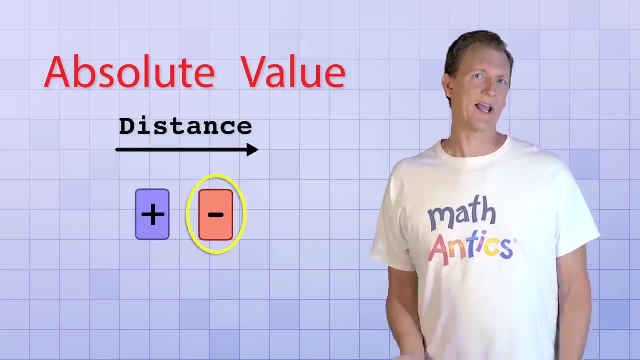 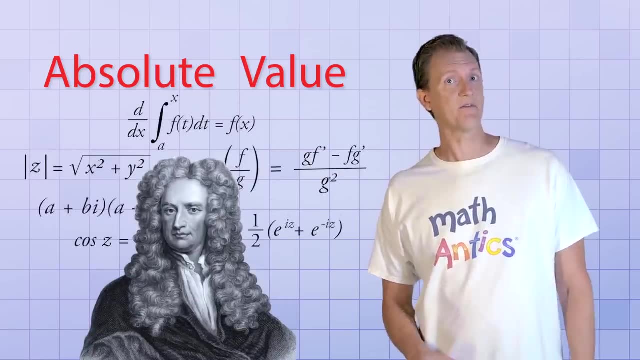 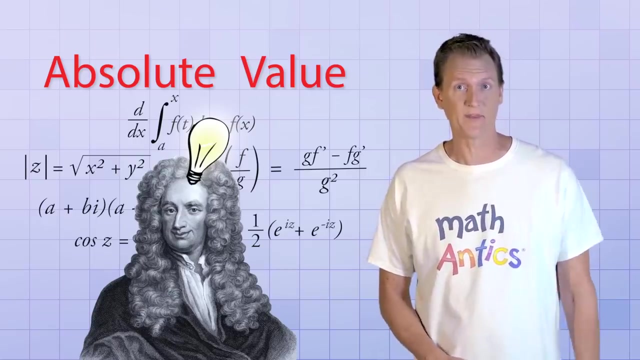 It's usually introduced in basic math right after you learn about negative numbers, But absolute value is a concept that's even more useful and more interesting in advanced math. Because of that, I'm going to teach you about absolute value using an idea that you usually don't encounter until a little later on in your math journey, And that idea 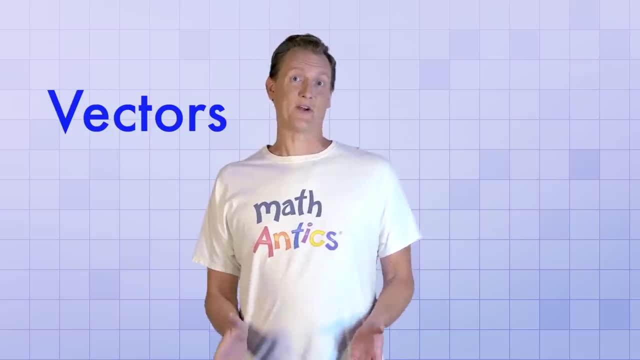 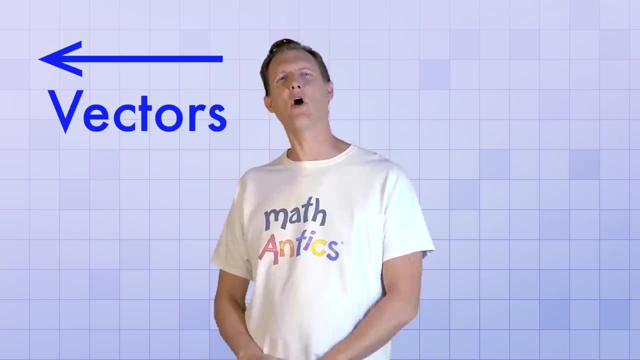 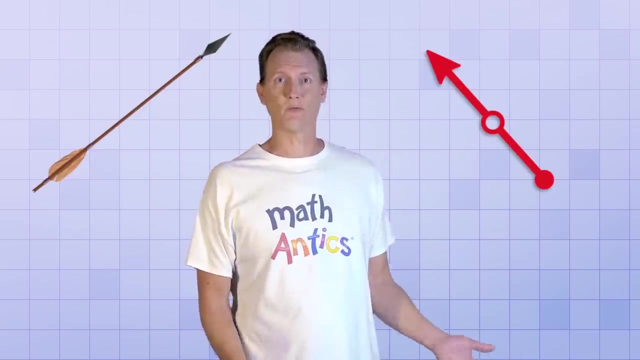 is vectors. The term vector might sound kinda technical, but they're actually really simple. Vectors are basically just arrows. In real life, an arrow can have all sorts of different properties. For example, this arrow is made of wood and has feathers, while this arrow is red plastic. 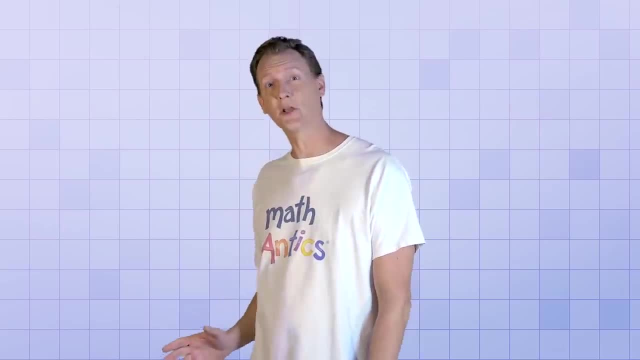 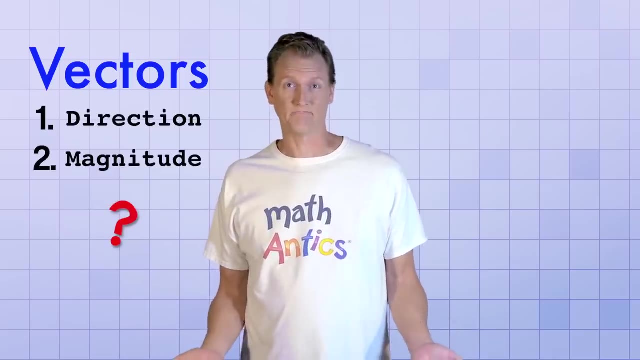 with a round thingy at the end. But in math, the arrows we call vectors only have two properties: They have a direction and a magnitude. What do those two properties mean? Well, direction is pretty obvious. It's just which way the arrow is pointing. 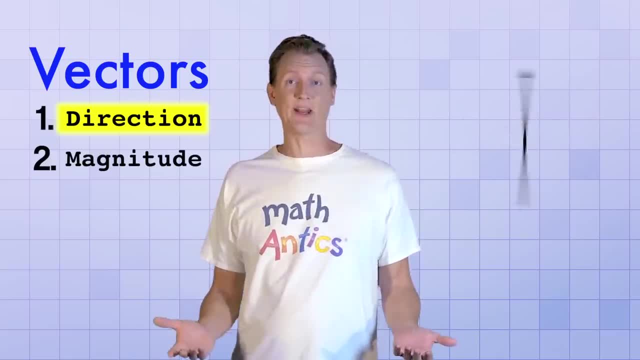 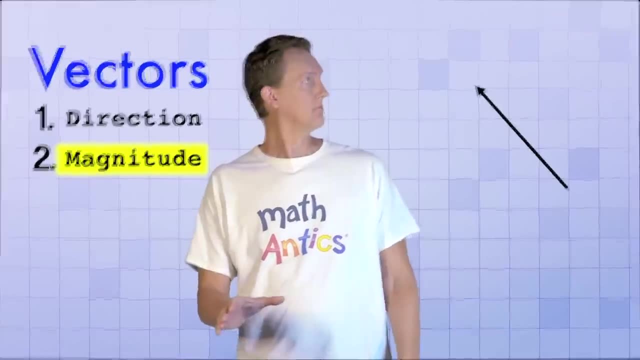 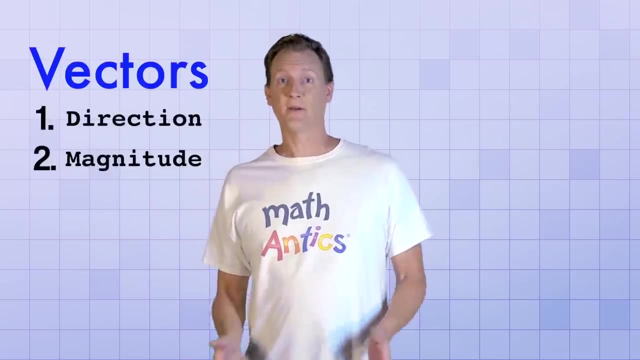 It could be up down, left, right or just about any direction you can think of. What does magnitude mean? Well, that word might make you think of an earthquake. Whew, Actually, magnitude is just a fancy word for the amount, extent or strength of something. 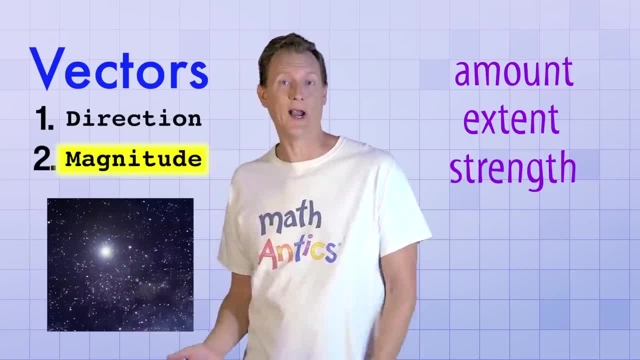 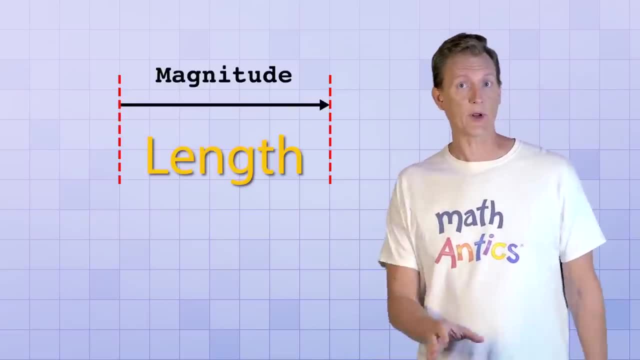 Like how strong an earthquake is Or how bright a star is or how heavy an object is. In the case of a vector, you can think of magnitude as being the length of the arrow. To see what I mean, let's use the number line to measure some vectors. 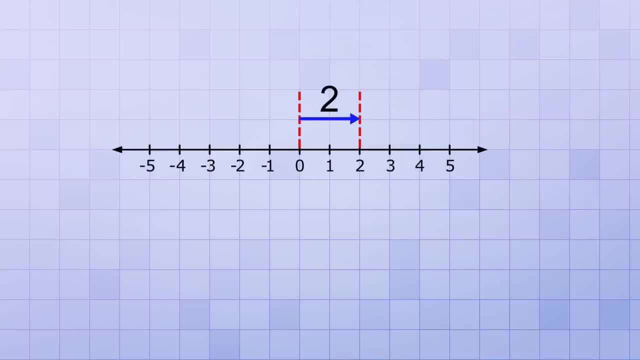 This vector has a magnitude or length of 2, because it starts at 0 and ends at 2.. And this vector has a magnitude or length of 5, because it starts at 0 and goes to 5.. 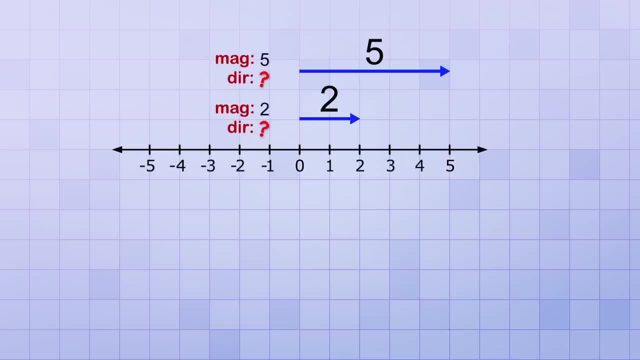 OK, so we know the magnitudes of these vectors, but what about their directions? Well, they're both pointing to the right on your screen And since we're using the number line as our reference, they're pointing in the positive direction, right? 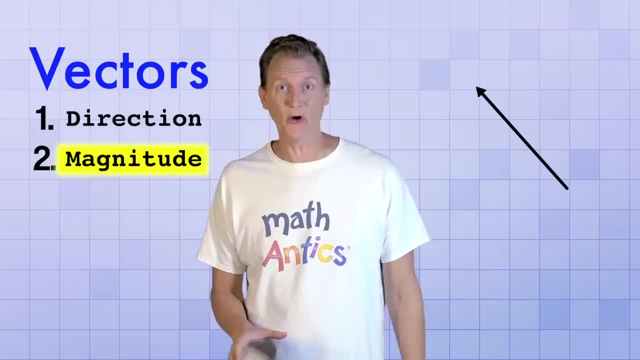 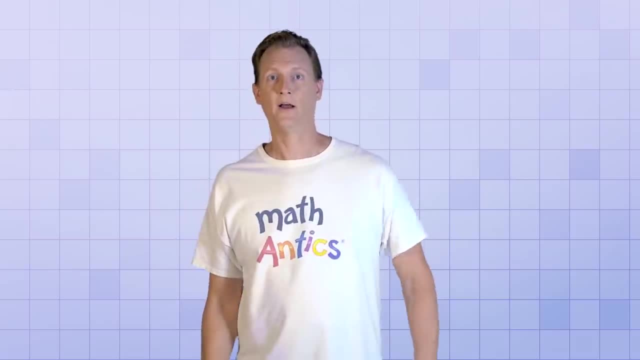 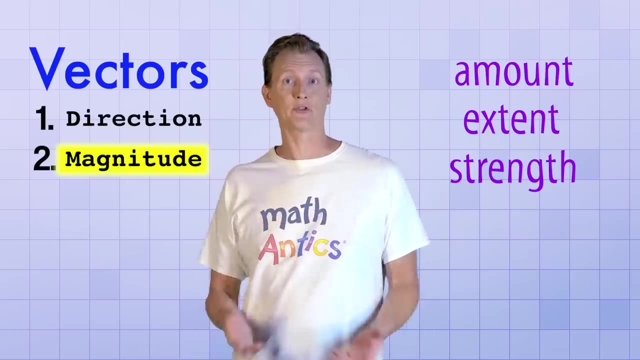 But what does magnitude mean? Well, that word might make you think of an earthquake. Actually, magnitude is just a fancy word for the amount, extent or strength of something, Like how strong an earthquake is Or how bright a star is. 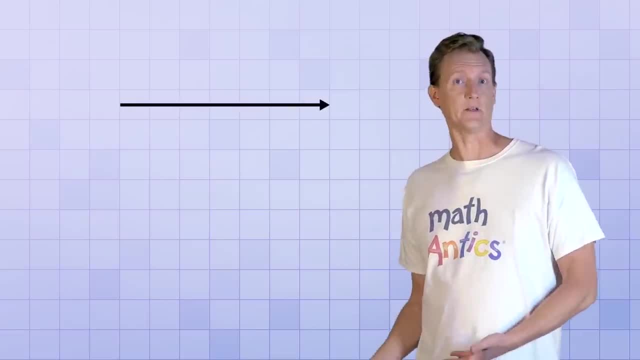 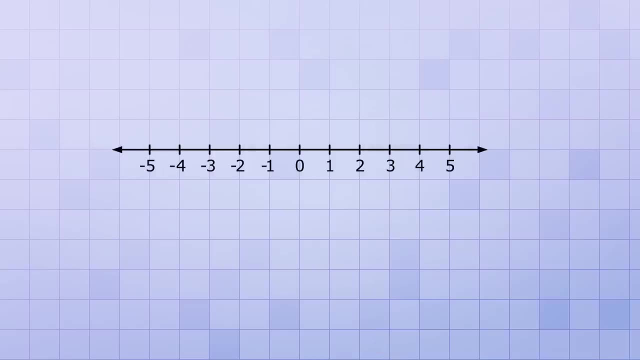 Or how heavy an object is. In the case of a vector, you can think of magnitude as being the length of the arrow. To see what I mean, let's use the number line to measure some vectors. This vector has a magnitude or length of 2, because it starts at 0 and ends at 2.. 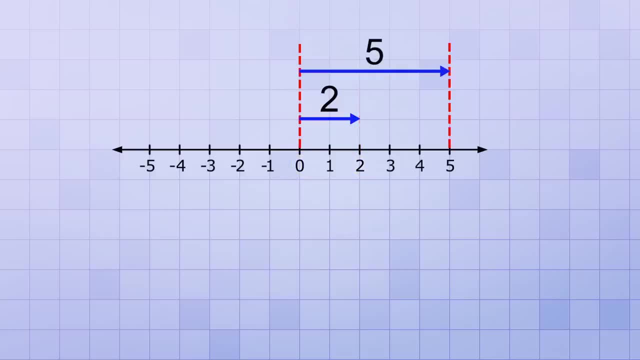 And this vector has a magnitude or length of 5, because it starts at 0 and goes to 5.. OK, so we know the magnitudes of these vectors, but what about their directions? Well, they're both pointing to the right on your screen. 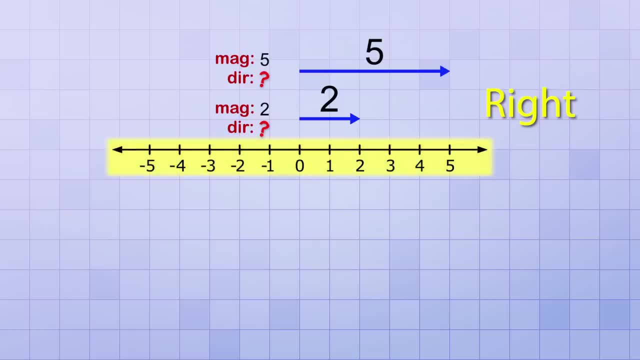 And since we're using the number line as our reference, they're pointing in the positive direction. right, But what about this vector here? It starts at 0,, like our other vectors do, but it ends at negative 2. And the arrow indicates that it's pointing in the exact opposite direction from the other two vectors. 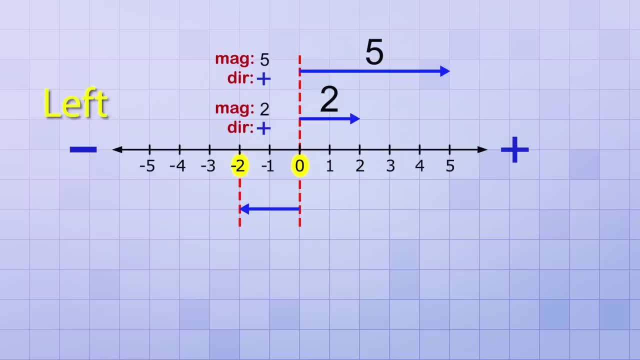 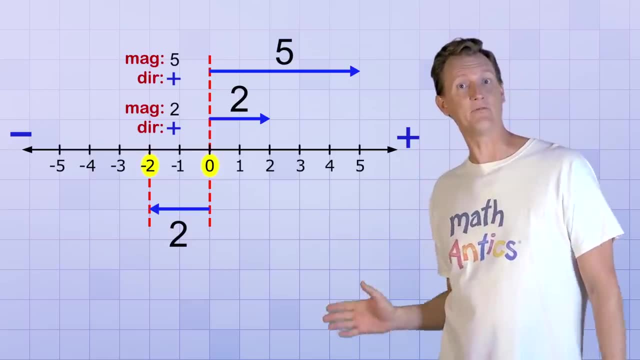 It's pointing to the left or in the negative direction of the number line. So what do you think its magnitude is For those of you that said 2,? you're right. Even though the vector is pointing in the negative direction, its length is still a positive number. 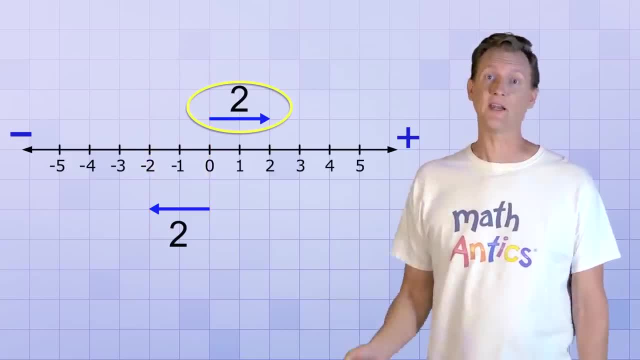 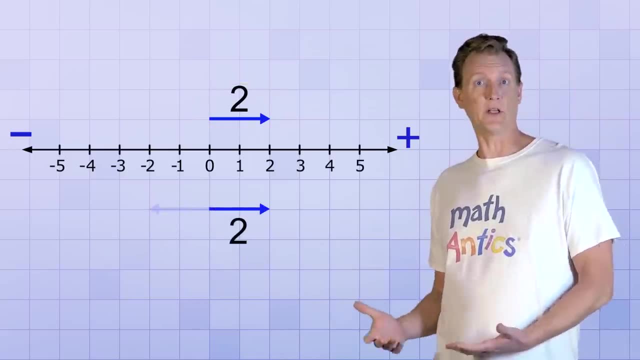 Its length is 2, just like this vector that's pointing in the positive direction. They're pointing in opposite directions, but if you rotate one vector around, you can see that they really do have the same length or magnitude. And another way to say that is that they have the same absolute value. 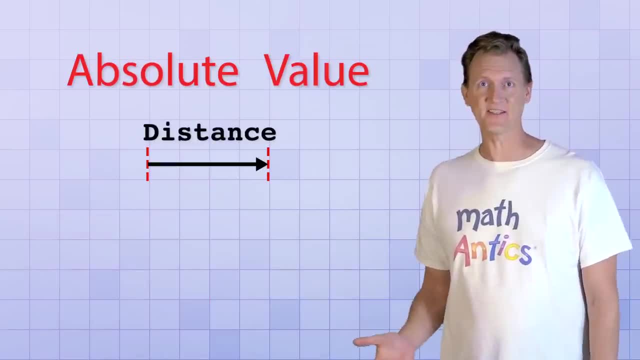 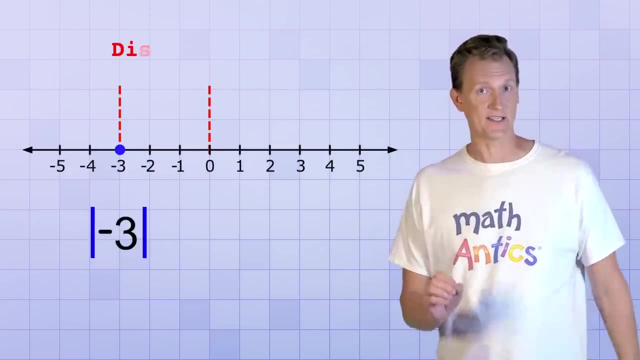 Ah, see why I said that absolute value has more to do with distance. In fact, when it comes to any number that you'd find on the number line, you can think of its absolute value as its distance from 0. This explains why absolute value is a little bit boring when you first learn about it. 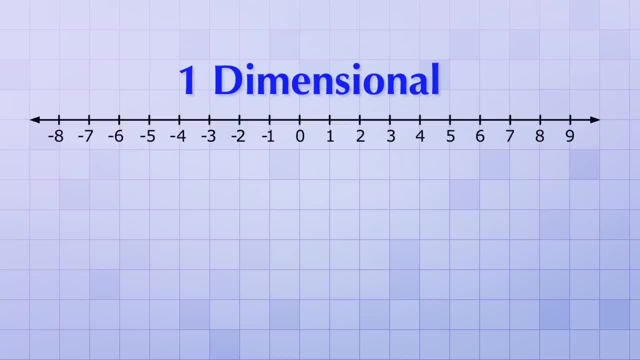 Because the number line is a one-dimensional space. there are only two possible directions: positive or negative. If you ask for the absolute value of any positive number along that line, you're asking for the distance that number is from 0,, which is just the number itself. 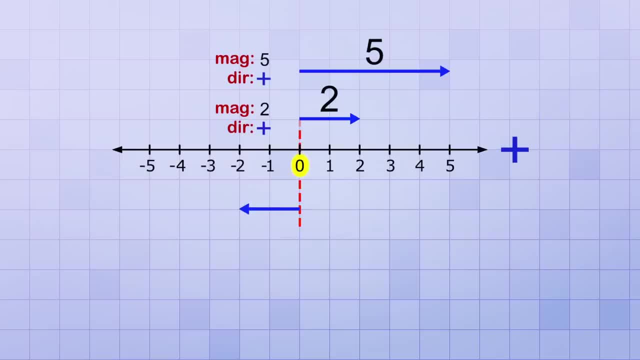 But what about this vector here? It starts at 0,, like our other vectors do, but it ends at negative 2.. And the arrow indicates that it's pointing in the exact opposite direction from the other two vectors. It's pointing to the left or in the negative direction of the number line. 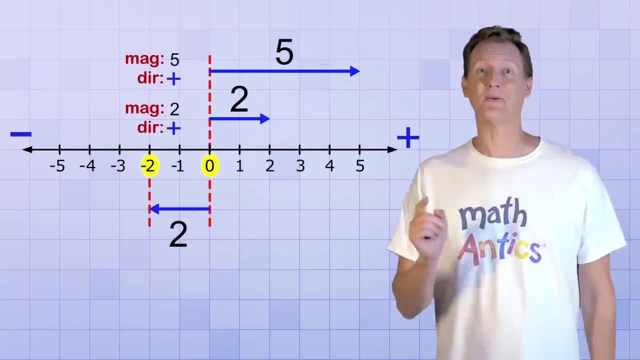 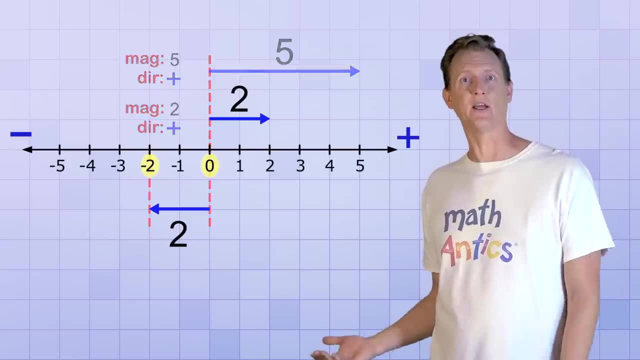 So what do you think its magnitude is? For those of you that said 2,? you're right. Even though the vector is pointing in the negative direction, its length is still a positive number. Its length is 2,, just like this vector that's pointing in the positive direction. 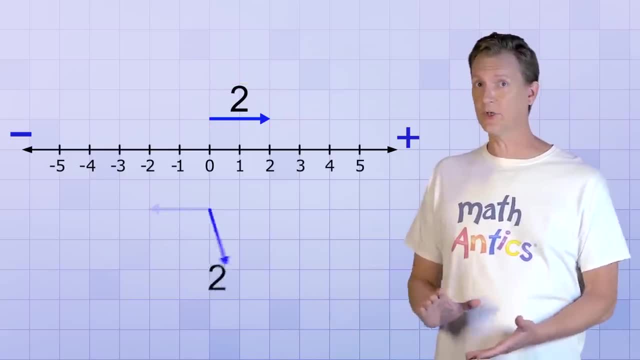 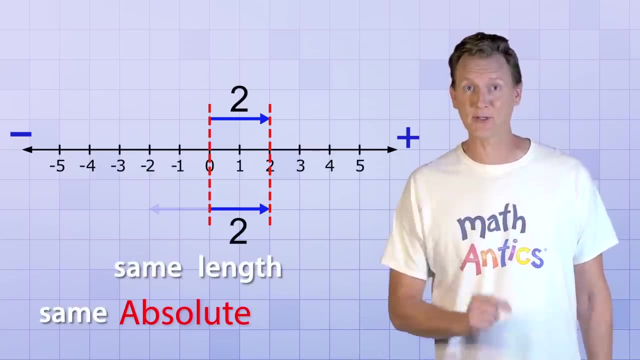 They're pointing in opposite directions, But if you rotate one vector around, you can see that they really do have the same length or magnitude. And another way to say that is that they have the same absolute value. Ah, see why I said that absolute value has more to do with distance. 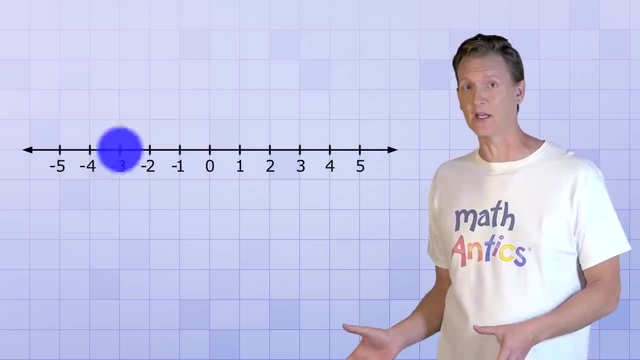 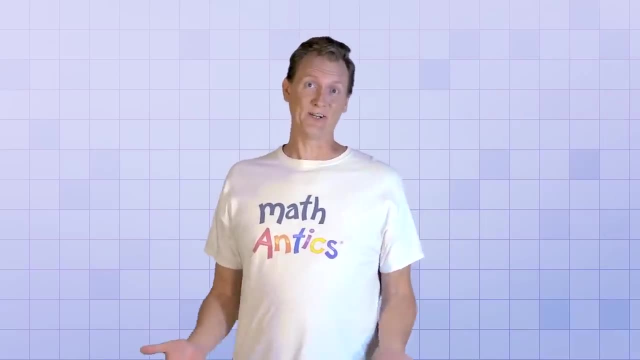 In fact, when it comes to any number that you'd find on the number line, you can think of its absolute value as its distance from 0. That explains why absolute value is a little bit boring when you first learn about it, Because the number line is a one-dimensional space. 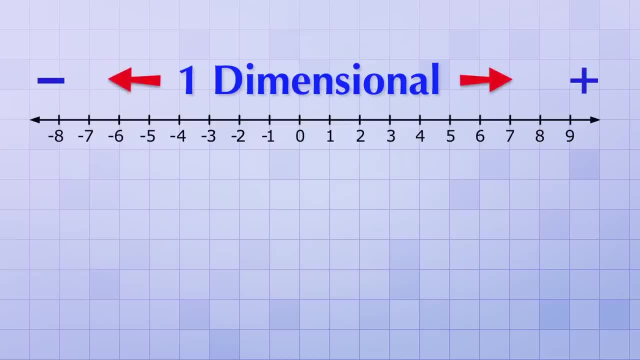 there are only two possible directions: positive or negative. If you ask for the absolute value of any positive number along that line, you're asking for the distance that number is from 0, which is just the number itself. And since the negative numbers are a mirror image of their positive counterparts, 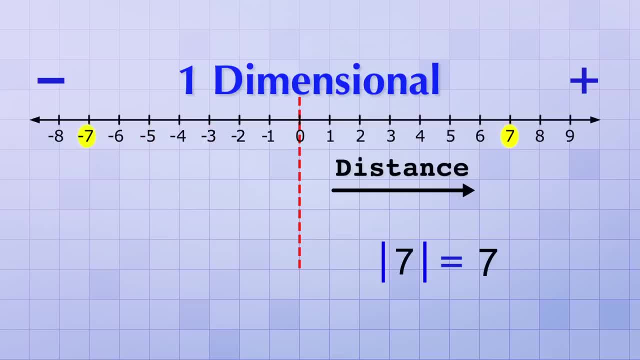 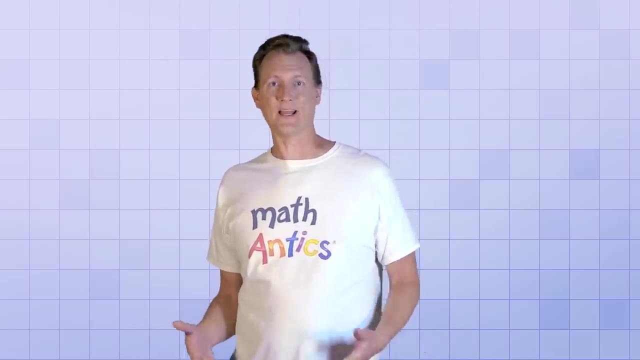 when you ask for the absolute value of any negative number along that line, the only difference is the direction or sign of that number, And that's why the absolute value of a negative number is just its positive counterpart. Hopefully that seems a little more interesting than just thinking about absolute value. 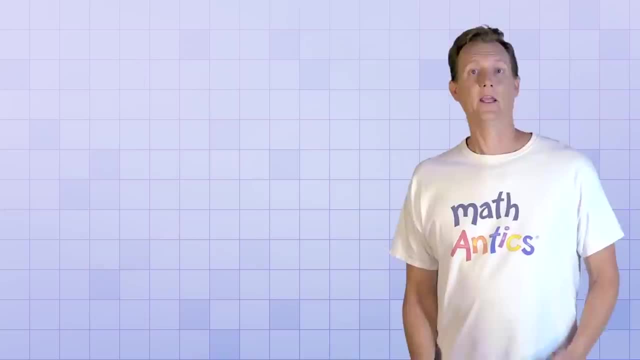 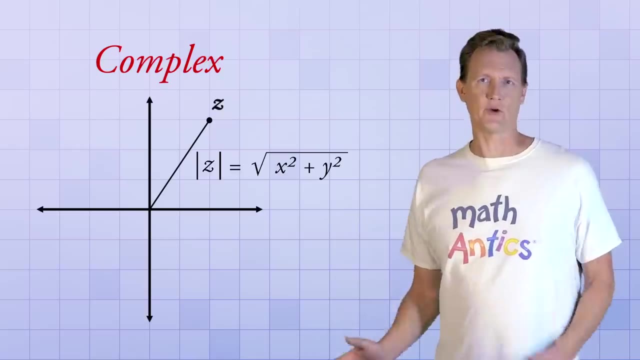 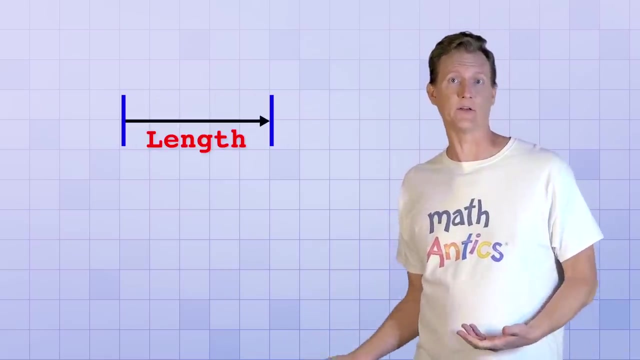 as a way to turn negative numbers into positive ones. In advanced math absolute value gets even more interesting and it actually gets kind of complex. Vectors can point in all sorts of directions besides just positive or negative. But hopefully thinking about absolute value as the magnitude or length of a vector makes it a little more interesting. 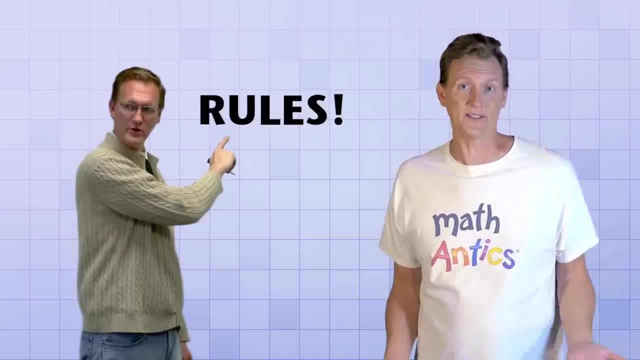 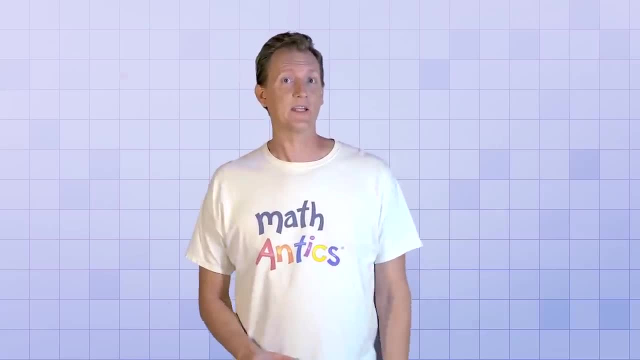 and it shows you that absolute value isn't just some silly rule that someone made up to make math even harder. And now that you know that absolute value is related to distance, it will help you understand a useful application of absolute value in the realm of basic math. 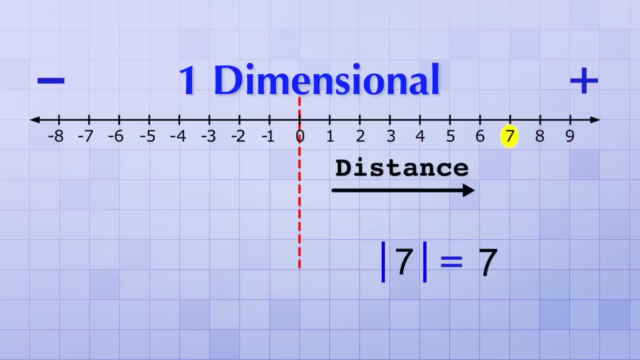 And since the negative numbers are a mirror image of their positive counterparts, when you ask for the absolute value of any negative number along the line, the only difference is the direction or sign of that number, And that's why the absolute value of a negative number is just its positive counterpart. 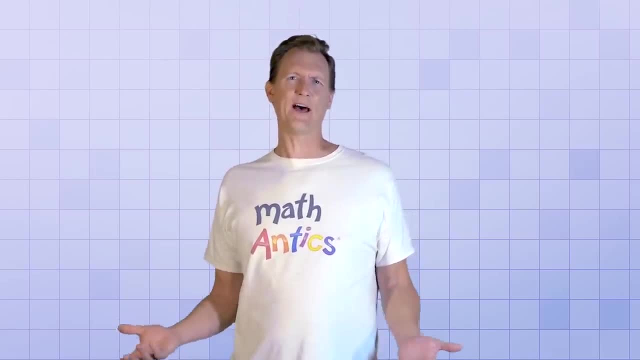 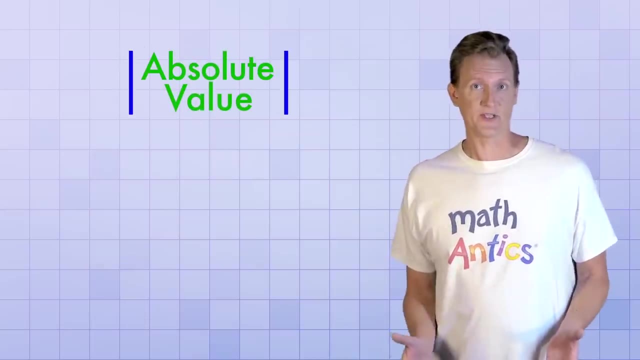 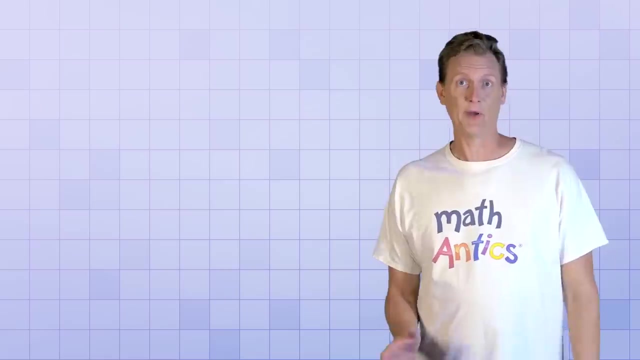 Hopefully that seems a little more interesting than just thinking about absolute value as a way to turn negative numbers into positive ones. In advanced math absolute value gets even more interesting And it actually gets kind of complex. Vectors can point in all sorts of directions besides just positive or negative. 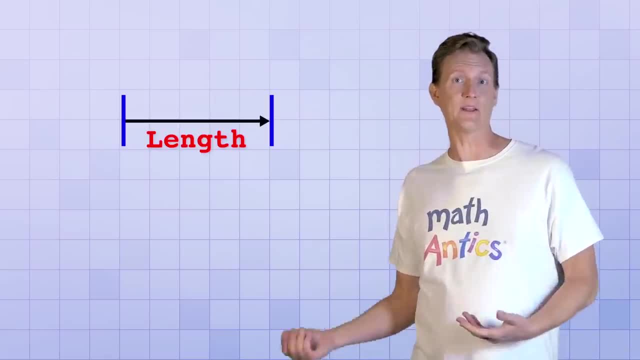 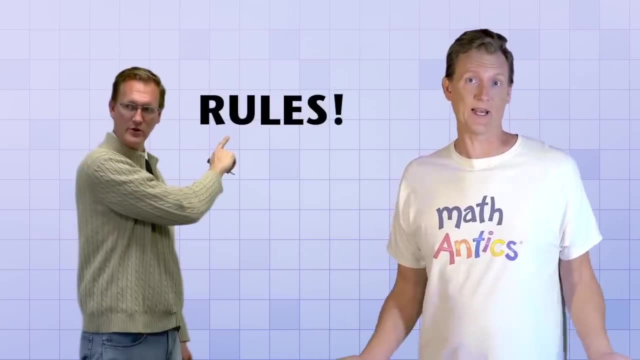 But hopefully, thinking about absolute value as the magnitude or length of a vector makes it a little more interesting and it shows you that absolute value isn't just some silly rule that someone made up to make math even harder. And now that you know that absolute value is related to distance, 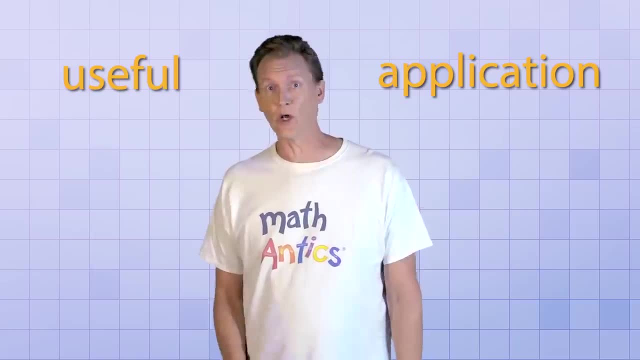 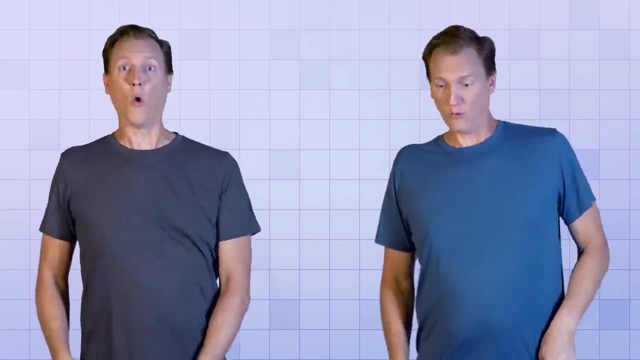 it will help you understand a useful application of absolute value in the realm of basic math. To see what I mean, suppose that you and your best friend each have a certain amount of money in your pockets and one of you has more than the other. 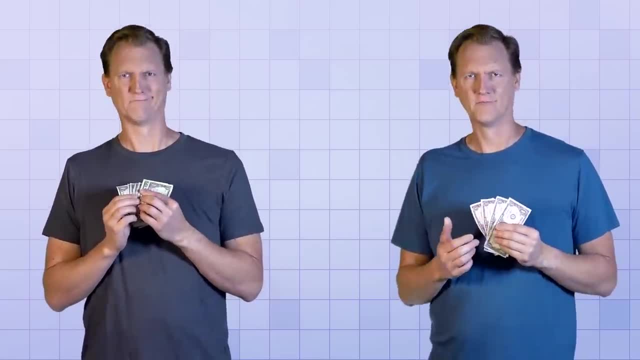 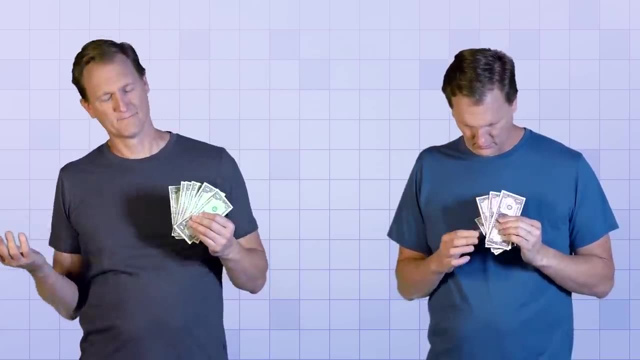 Now, it doesn't really matter to you who has more money, you just want to know the difference between the amounts. How do you find the difference between two amounts? Yep, you subtract them, And the answer you get from subtracting depends on the order of the numbers. 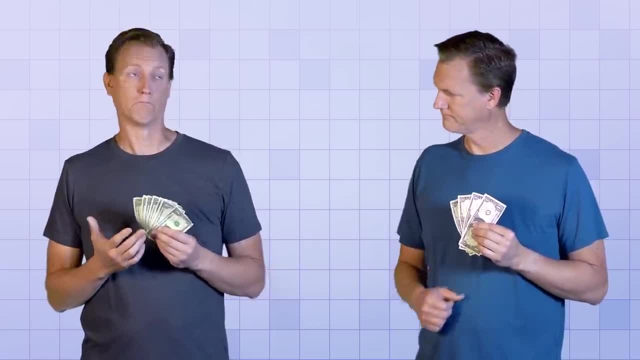 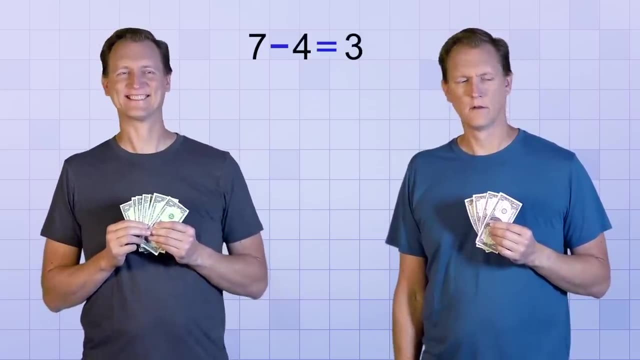 because subtracting doesn't have the commutative property right. If we subtract the amounts in this order: 7 minus 4, we'll get the answer 3.. But if we subtract the amounts in this order: 4 minus 7, we'll get the answer negative 3.. 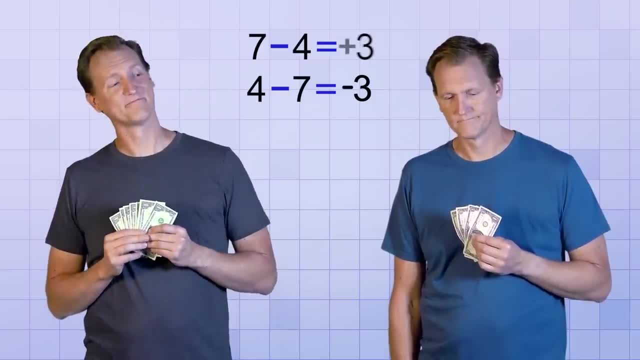 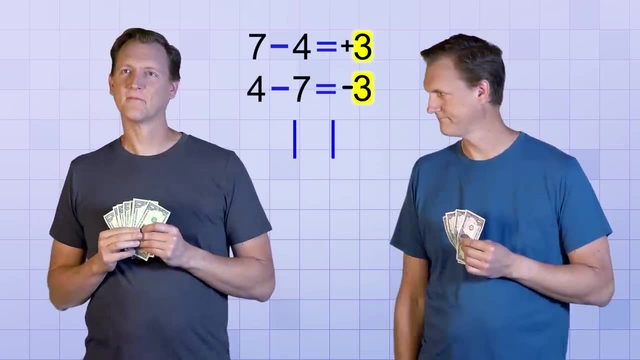 Do you notice something about these answers? Yep, Even though the sign or direction is different, the magnitudes are the same. They're both 3.. That means that the absolute values of the answers would be the same And, like I said, we don't really care who has more money. we just want to know how much that difference is. 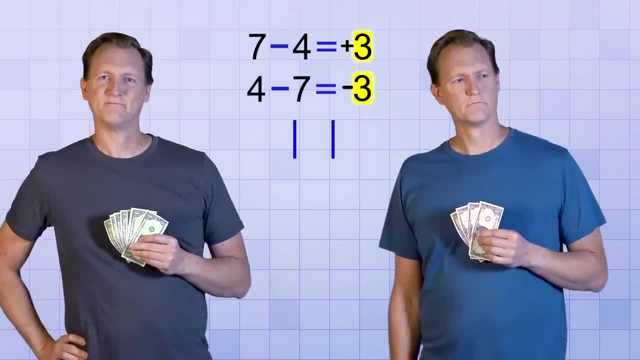 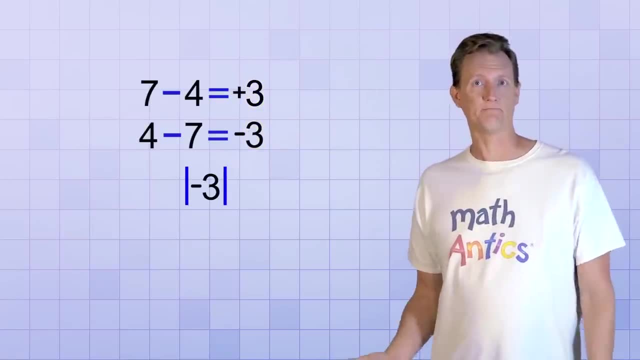 So in this problem we only need the magnitude or absolute value of the difference. No matter which way we do the subtraction, we just take the absolute value of the answer to get what we want, And this idea can be really helpful when you're entering numbers into your calculator. 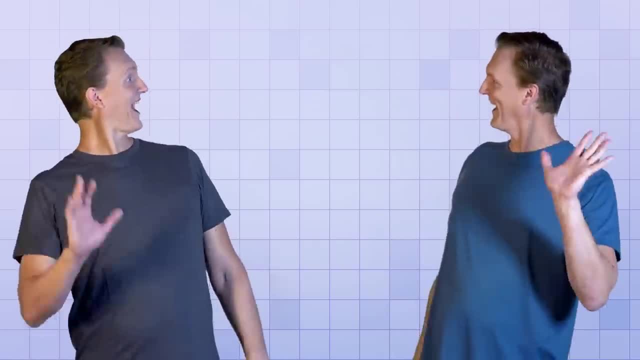 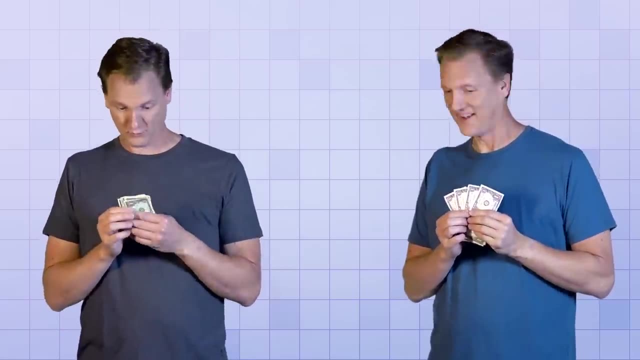 To see what I mean. suppose that you and your best friend each have a certain amount of money in your pockets, and one of you has more than the other. Now, it doesn't really matter to you who has more money, but you want to know the difference between the amounts. 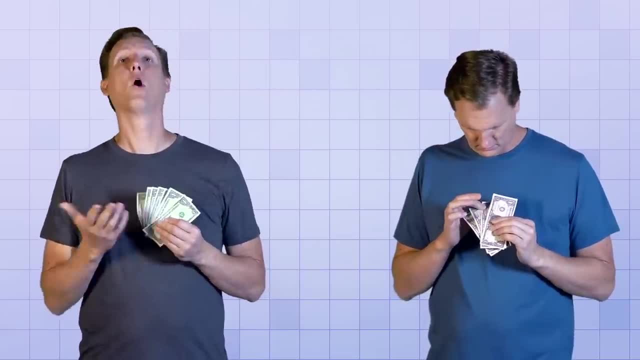 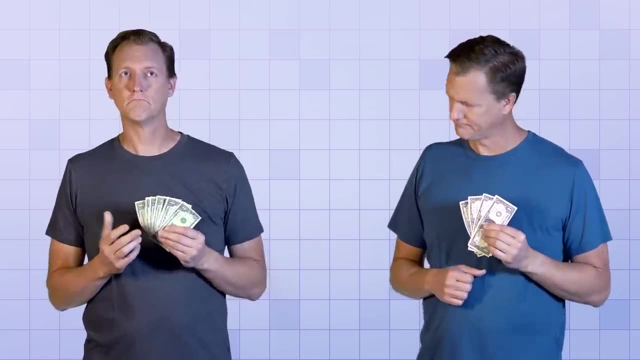 How do you find the difference between two amounts? Yep, you subtract them, And the answer you get from subtracting depends on the order of the numbers, because subtracting doesn't have the commutative property, right? If we subtract the amounts in this order- 7 minus 4, we'll get the answer 3.. 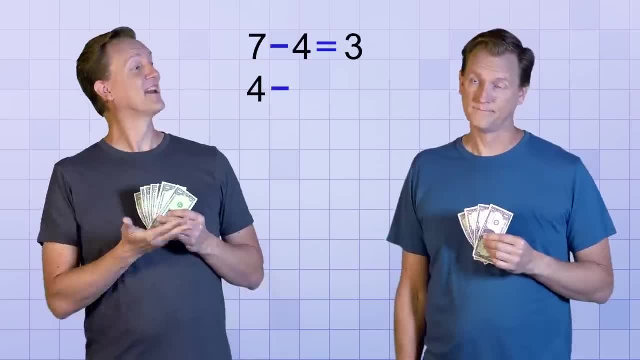 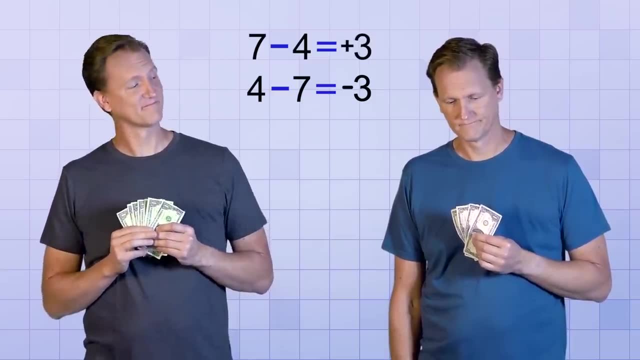 But if we subtract the amounts in this order, 4 minus 7, we'll get the answer negative 3.. Do you notice something about these answers? Yep, Even though the sign or direction is different, the magnitudes are the same. 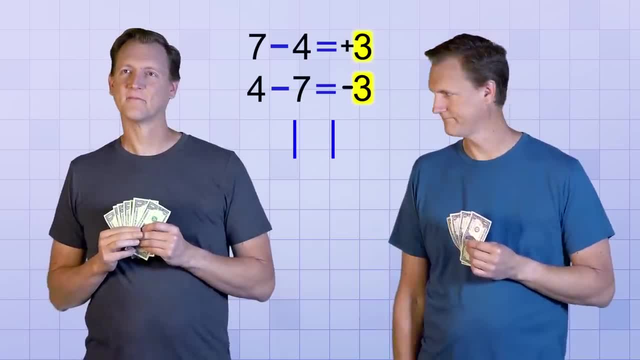 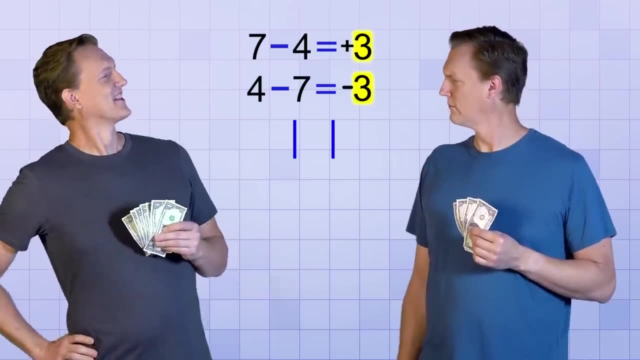 They're both 3.. That means that the absolute values of the answers would be the same And, like I said, we don't really care WHO has more money, we just want to know how much that difference is. So in this problem, we only need the magnitude or absolute value of the difference. 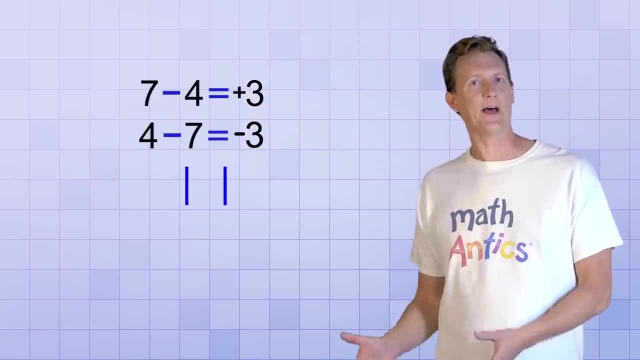 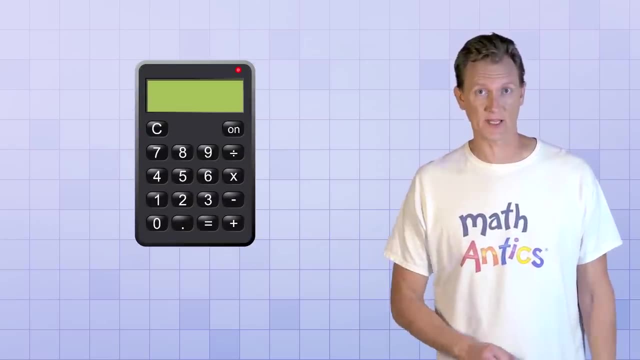 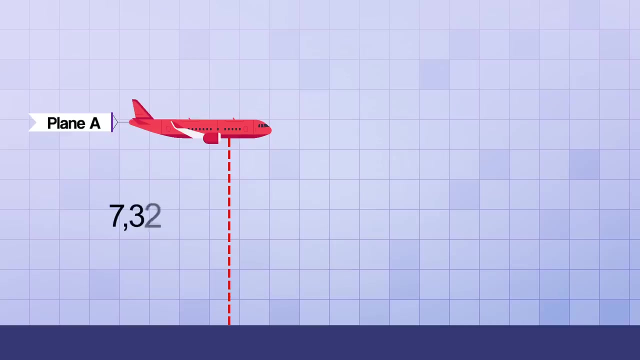 No matter which way we do the subtraction, we just take the absolute value of the answer to get what we want, And this idea can be really helpful when you're entering numbers into your calculator to solve math problems like this one. Let's say an airplane is flying at an altitude of 7,328 meters. 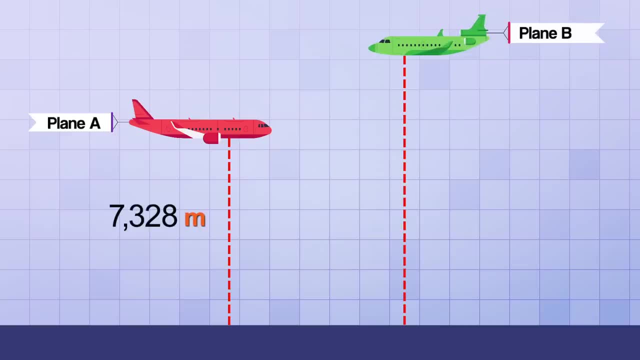 and another plane is flying at an altitude of 9,150 meters And the problem asks you to find the difference in their altitudes. You know that means you need to subtract. so you quickly get out your calculator and start typing in the first number. 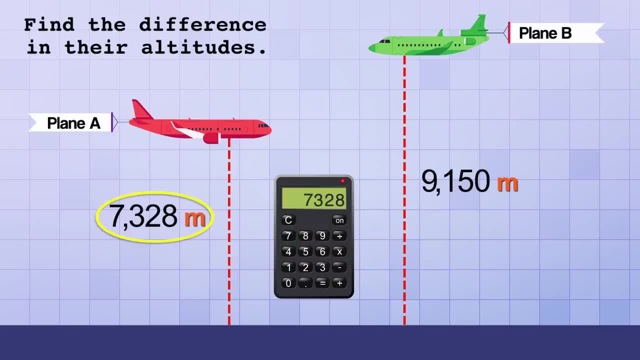 But as soon as you get the 7,328 entered and hit the subtract button, you realize the second altitude is bigger. That means you'll have a negative number as your answer. Should you start over and type the bigger number first? Thanks to absolute value, you don't have to. 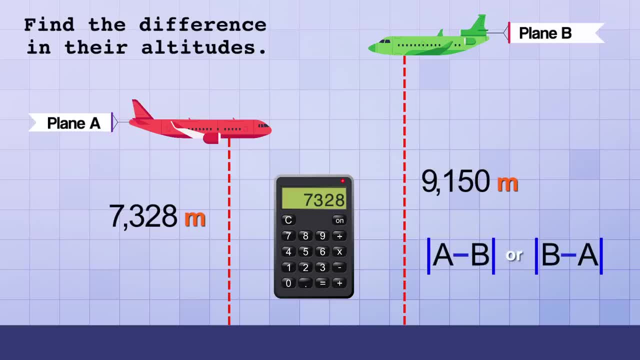 No matter which order you subtract, the numbers in, the magnitude of the answer will be the same, Just the direction or sign of the answer will be different. So if you continue on and enter 9,150 and then hit the equal sign, the answer you get is negative: 1,850. 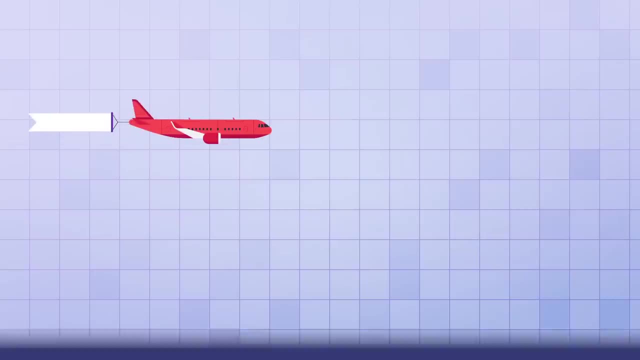 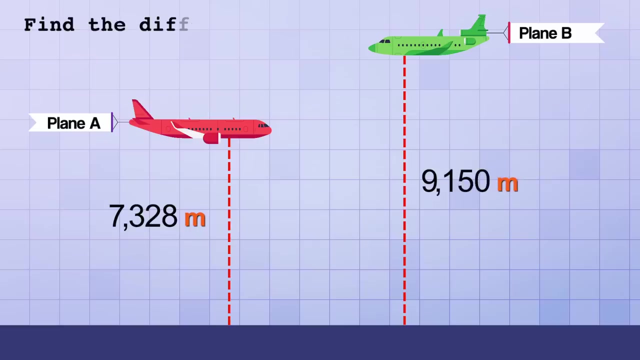 to solve math problems like this one. Let's say an airplane is flying at an altitude of 7,328 meters and another plane is flying at an altitude of 9,150 meters And the problem asks you to find the difference in their altitudes. 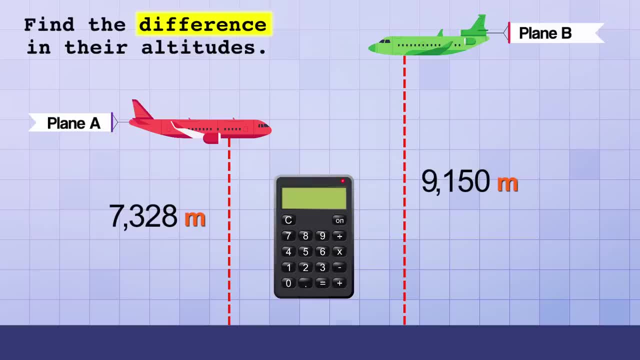 You know that means you need to subtract. so you quickly get out your calculator and start typing in the first number. But as soon as you get the 7,328 entered and hit the subtract button you realize the second altitude is bigger. That means you'll have a negative number as your answer. 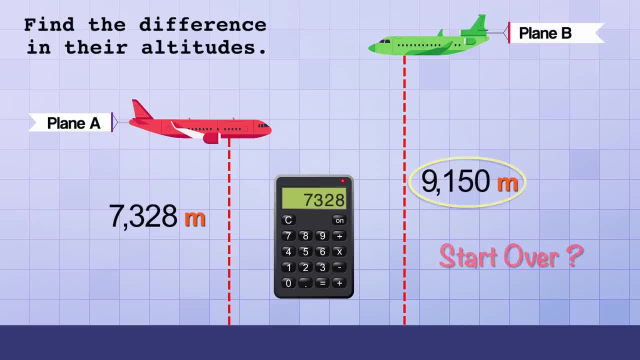 Should you start over and type the bigger number first? Thanks to absolute value, you don't have to. No matter which order you subtract the numbers in the magnitude of the answer will be the same, Just the direction or sign of the answer will be different. 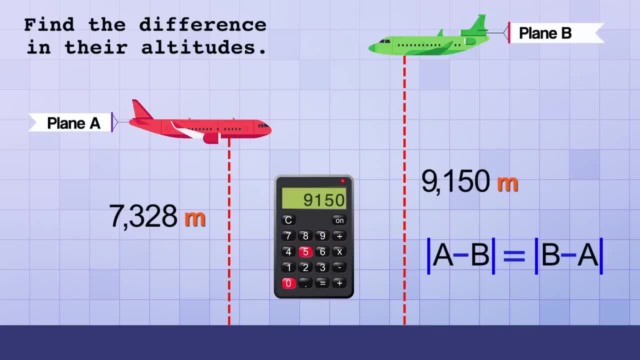 So if you continue on and enter 9,150 and then hit the equal sign, the answer you get is negative 1,822.. Now all you have to do is mentally think of that number as an absolute value and ignore the minus sign. 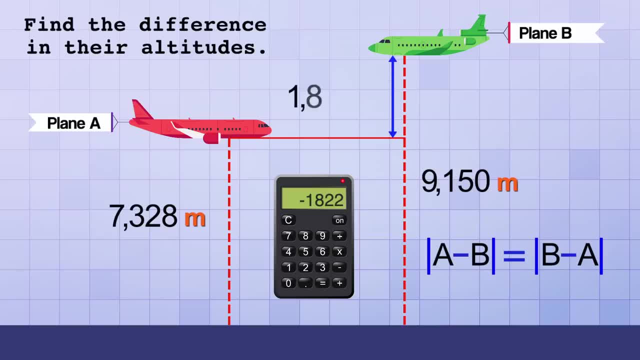 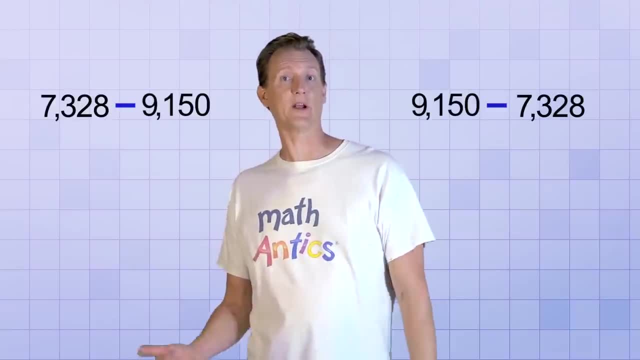 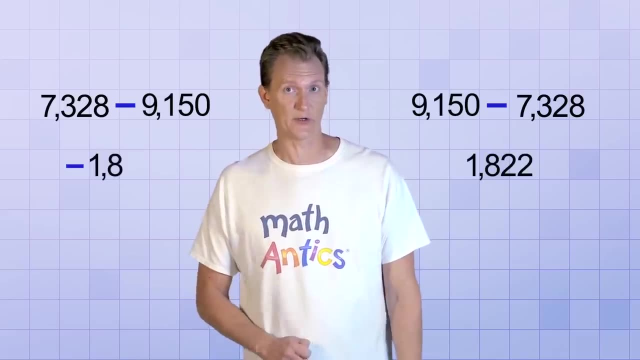 The difference in the altitudes of the two planes is 1,822 meters. If you're not quite convinced of that, try the problem for yourself, subtracting both ways, and see what answers you get. In one case you'll get 1,822 and in the other you'll get negative 1,822.. 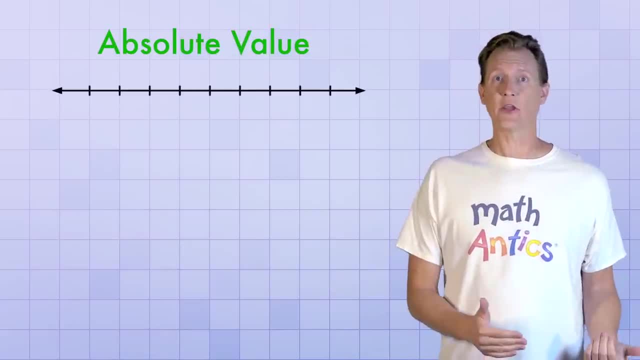 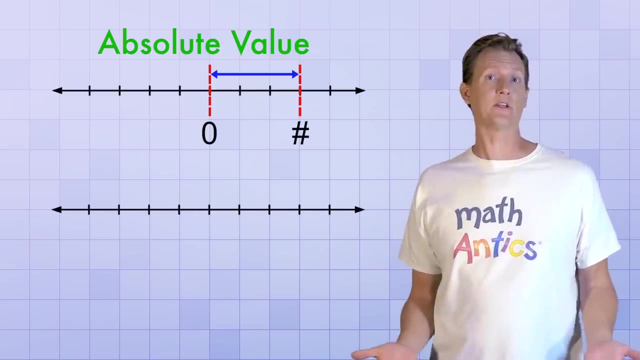 So now you know that, in its most basic form, absolute value is just the distance between a number and zero on the number line, And you've also seen how it can be helpful when you want to find the difference between two different numbers, regardless of which is greater. 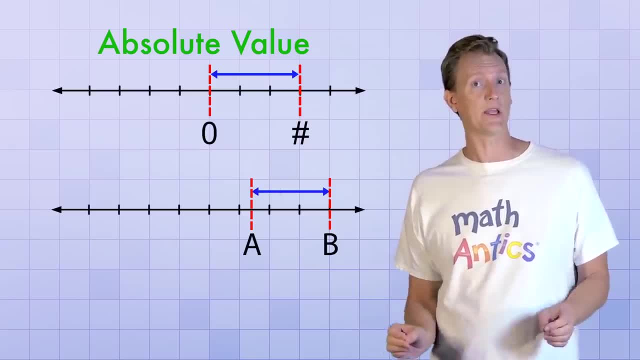 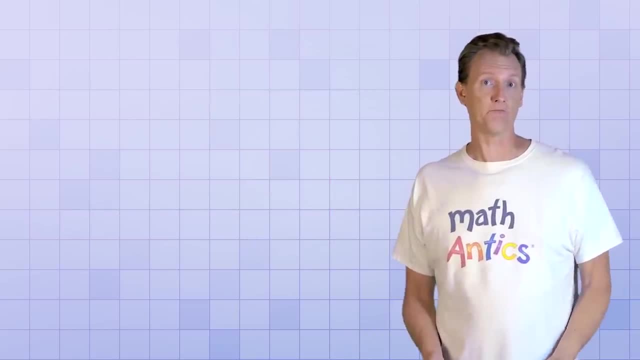 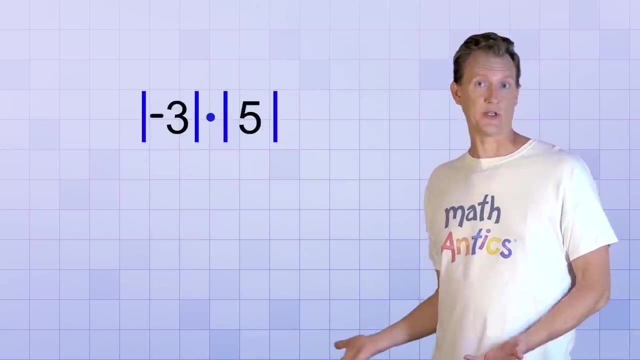 In that case, the absolute value represents the distance between those two numbers. The last thing I want to show you in this video is how to handle a couple situations involving absolute value that you might encounter on tests when evaluating mathematical expressions. For example, what if you're asked to evaluate this expression involving absolute values? 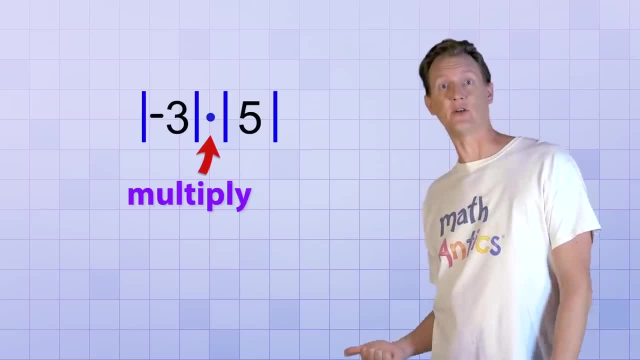 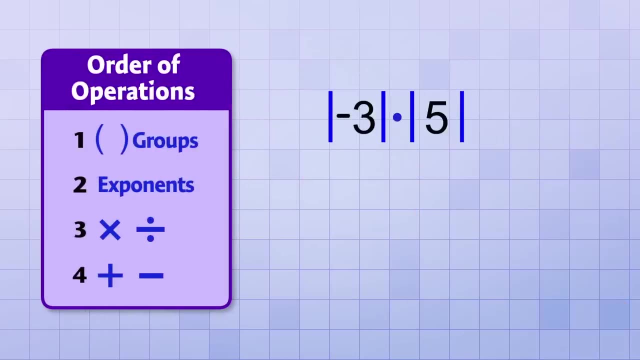 We learned how to multiply integers in the last video, but now these integers are inside absolute value signs. So what do we do? Well, when it comes to order of operations, absolute value signs are similar to parentheses, which means that you need to take care of them first before you start working on the other arithmetic operations. 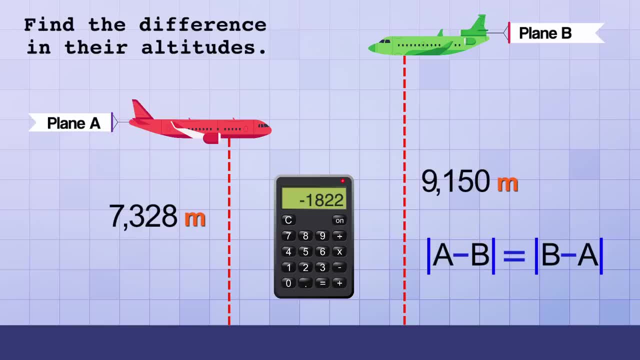 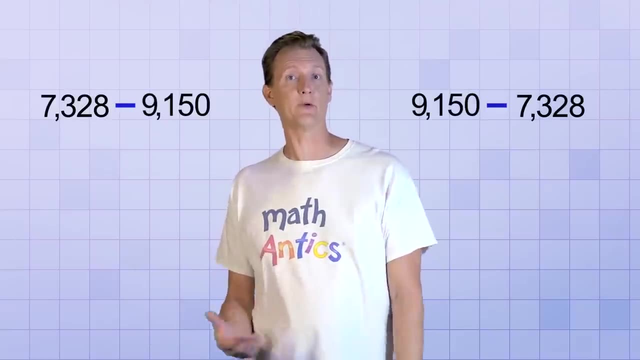 Now all you have to do is mentally think of that number as an absolute value and ignore the minus sign. The difference in the altitudes of the two planes is 1,822 meters. If you're not quite convinced of that, try the problem for yourself, subtracting both ways, and see what answers you get. 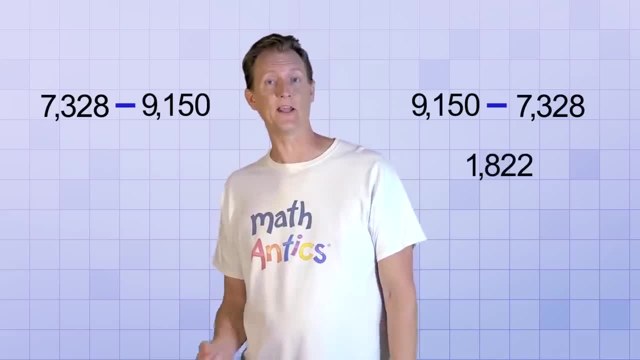 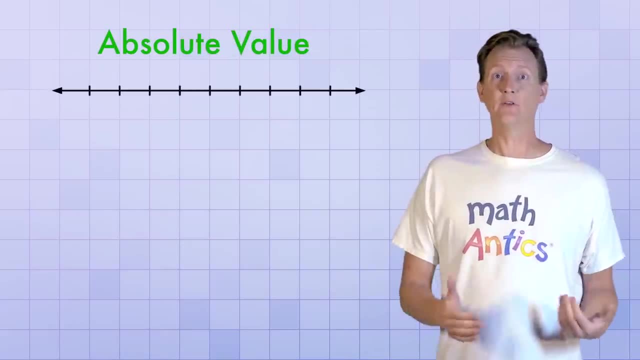 In one case you'll get 1,822 and in the other you'll get negative 1,822.. So now you know that, in its most basic form, absolute value is negative 1,822.. The absolute value is just the distance between a number and zero on the number line. 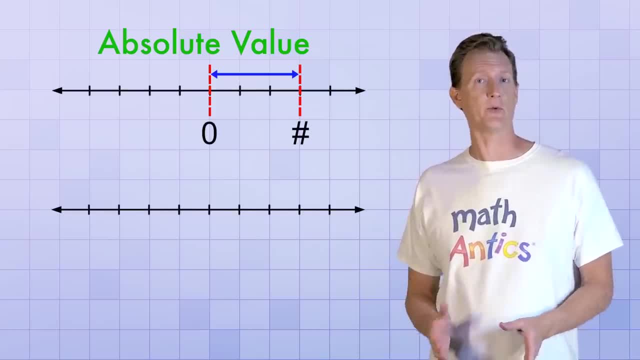 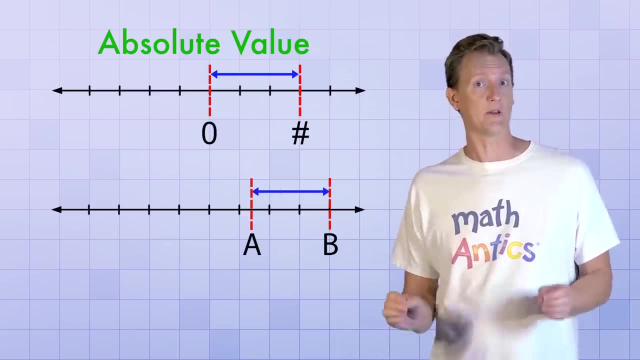 And you've also seen how it can be helpful when you want to find the difference between two different numbers, regardless of which is greater. In that case, the absolute value represents the distance between those two numbers. The last thing I want to show you in this video is how to handle a couple situations involving 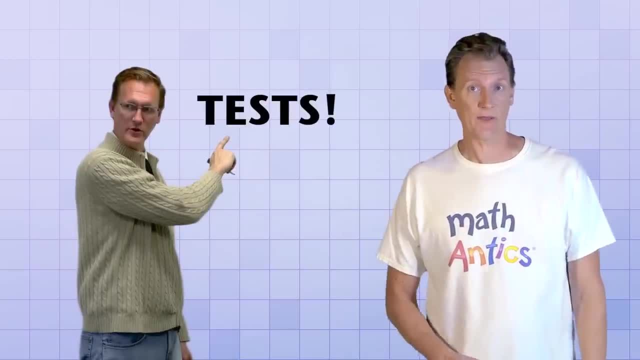 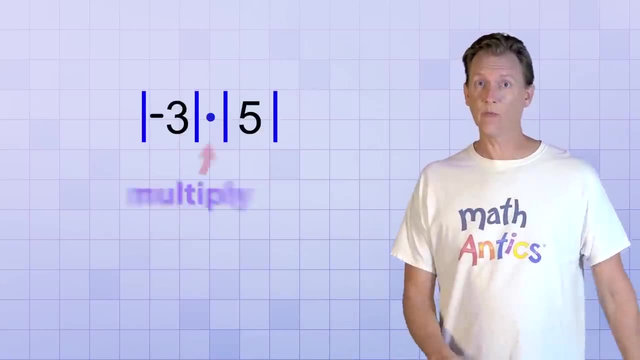 absolute value that you might encounter on tests when evaluating mathematical expressions, For example, what if you're asked to evaluate this expression involving absolute value? We learned how to multiply integers in the last video, but now these integers are inside absolute value signs, So what do we do? 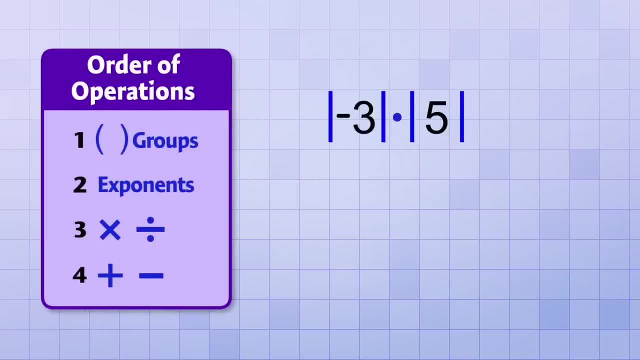 Well, when it comes to order of operations, absolute value signs are similar to parentheses, which means that you need to take care of them first before you start working on the other arithmetic operations. So, in this problem, before we can multiply the integers, 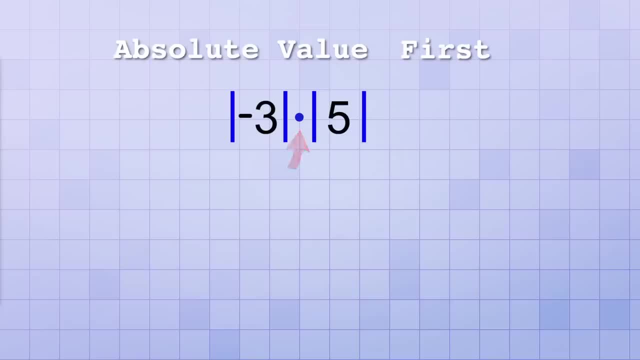 we need to take the absolute value of the numbers first. The absolute value of negative 3 is 3, and the absolute value of 5 is 3.. So the problem simplifies to 3 times 5,, which is 15.. 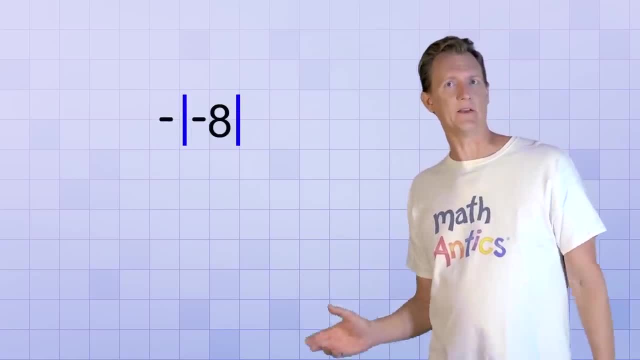 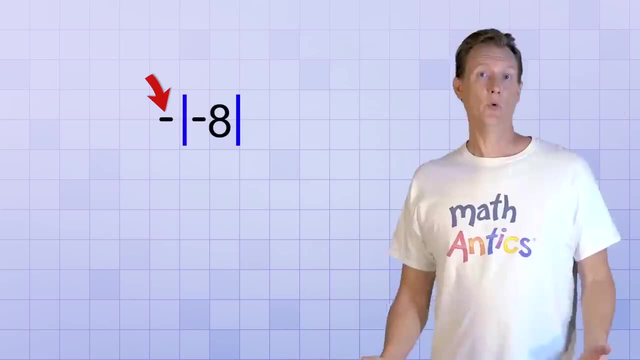 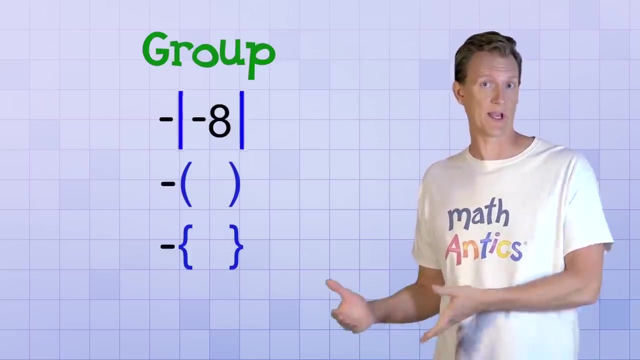 That example was pretty easy. but what about this one Negative absolute value of negative 8.. Why is there an extra negative sign outside of the absolute value signs? Well, whenever you see a negative sign immediately outside and to the left of a group, like parentheses, braces or the absolute value signs, 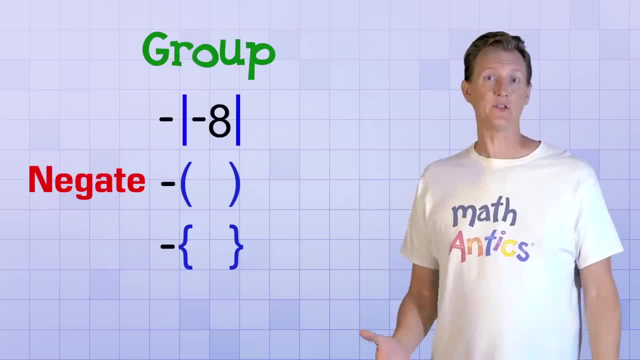 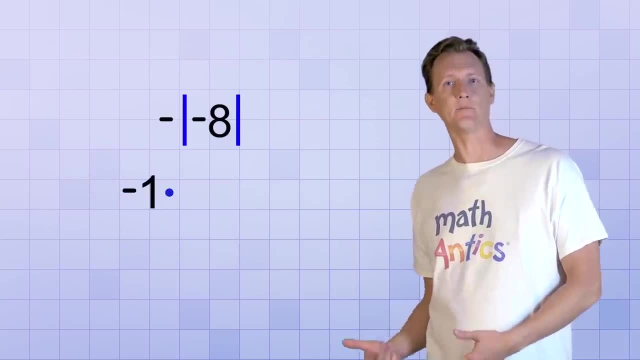 it means that you need to negate that group. That means you need to multiply that group by negative 1.. So, if it helps, you can think of this problem like this: Negative 1 times the absolute value of negative 8.. And since absolute value signs are groups like parentheses, 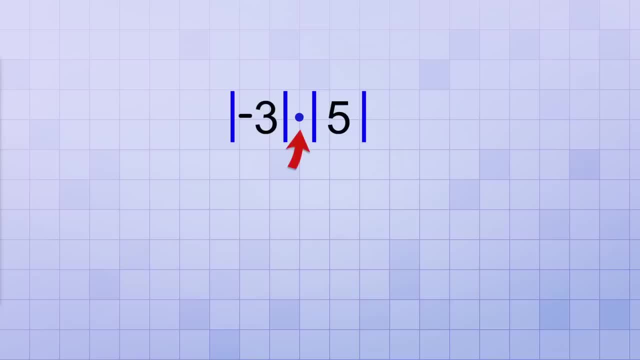 So in this problem, before we can multiply the integers, we need to take the absolute value of the numbers first. The absolute value of negative 3 is 3 and the absolute value of 5 is 5.. So the problem simplifies to 3 times 5, which is 15.. 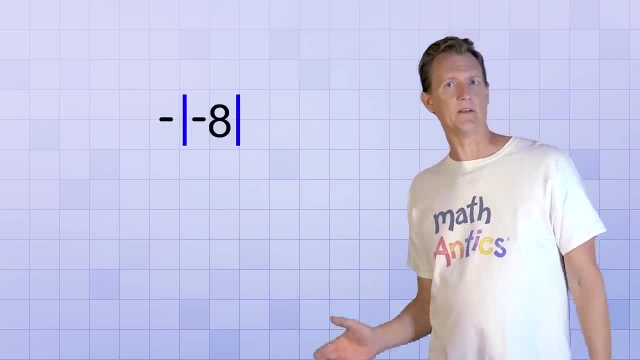 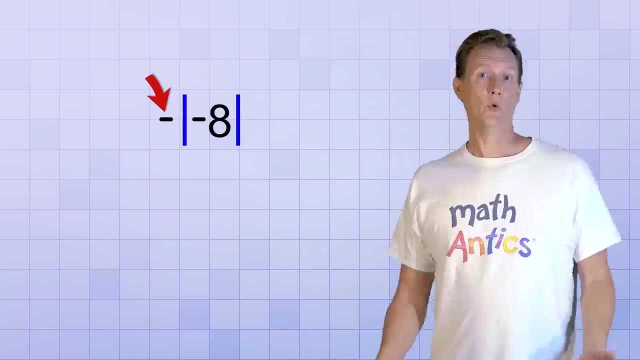 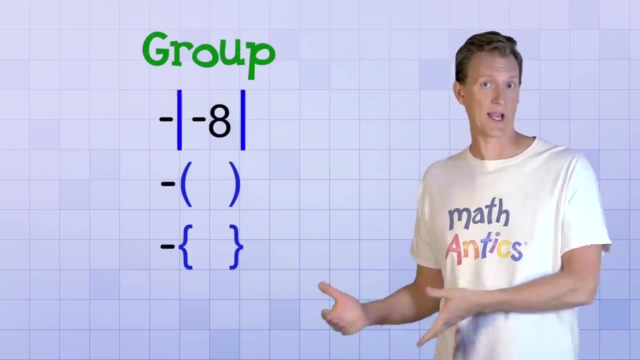 That example was pretty easy. but what about this one Negative absolute value of negative 8.. Why is there an extra negative sign outside of the absolute value signs? Well, whenever you see a negative sign immediately outside and to the left of a group, like parentheses, braces or the absolute value signs, 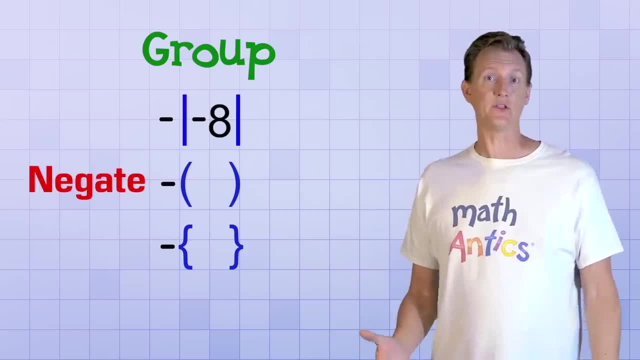 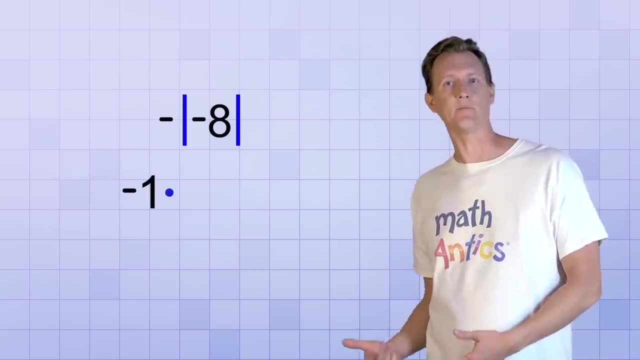 it means that you need to negate that group. That means you need to multiply that group by negative 1.. So, if it helps, you can think of this problem like this: Negative 1 times the absolute value of negative 8.. And since absolute value signs are groups like parentheses, to simplify it we would first need to do the absolute value. 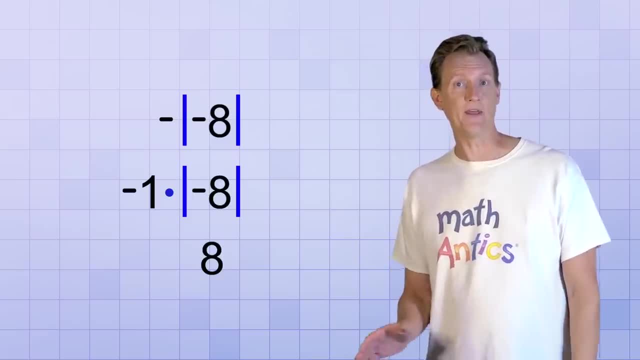 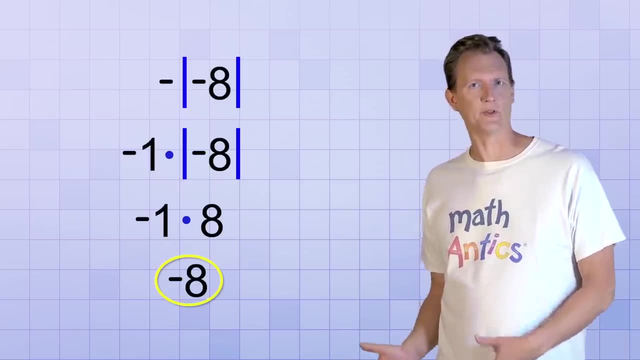 The absolute value of negative 8 is 8.. And then we multiply that by negative 1 and we get the answer negative 8.. That seems pretty simple too, But I want to use this example to point out an important difference between parentheses and absolute value signs. 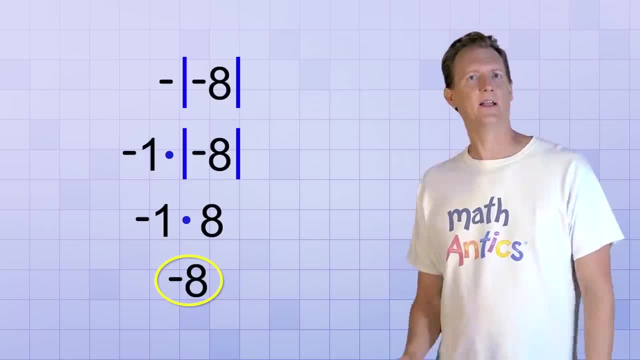 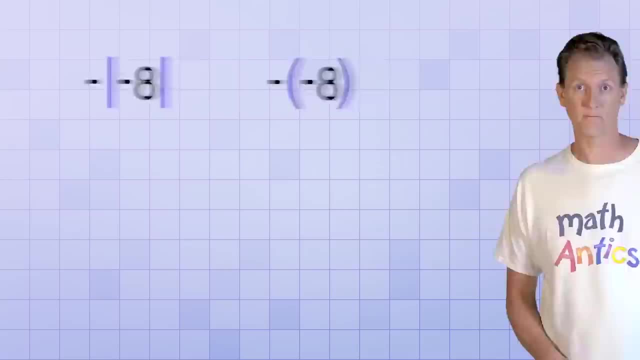 It's a difference that can trick you on a test if you're not careful. Let's see the expression we just simplified side by side with a similar expression that has parentheses instead of absolute value signs. In both of these cases, the negative sign outside the group is telling us to negate the group. 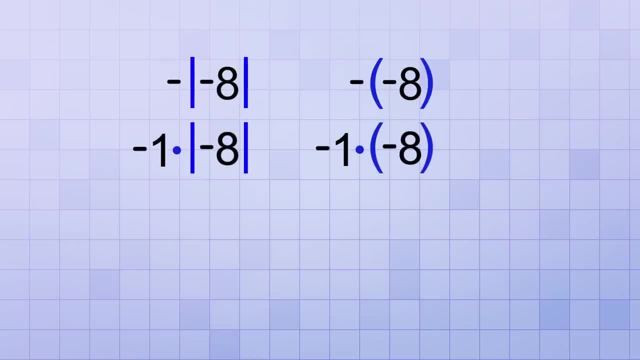 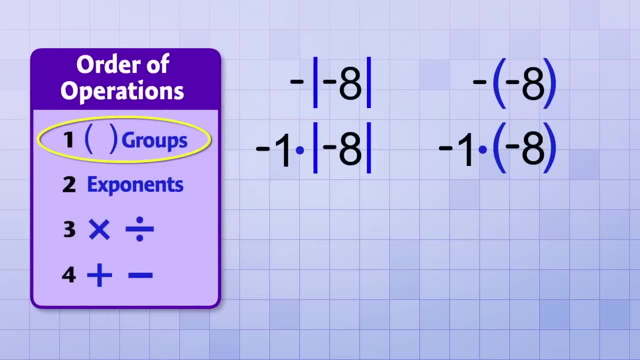 That means multiplying it by negative 1.. But there's a very important difference between the two expressions. The order of operations rules tells us to do things that are inside of groups first. right, But there's nothing to do inside the parentheses. It's just a negative 8 hanging out inside of them. 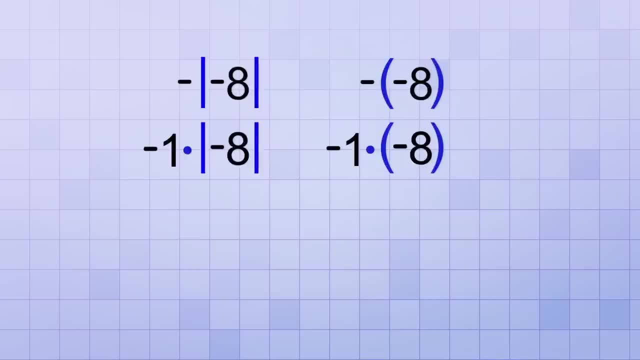 And the parentheses themselves don't tell us to do anything. So this expression is just asking us to multiply negative 1 times negative 8, which is positive 8.. But in the case of the absolute value signs, while they do function like groups, 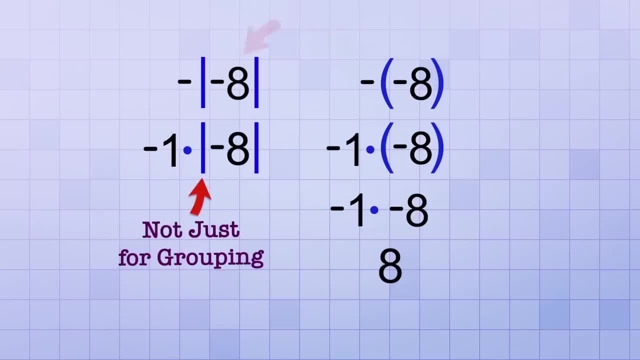 they aren't just for grouping, like the parentheses are. They're also telling us to do something to whatever is inside of them. What are they telling us to do? They tell us to use the magnitude of the number inside, which would be positive 8.. 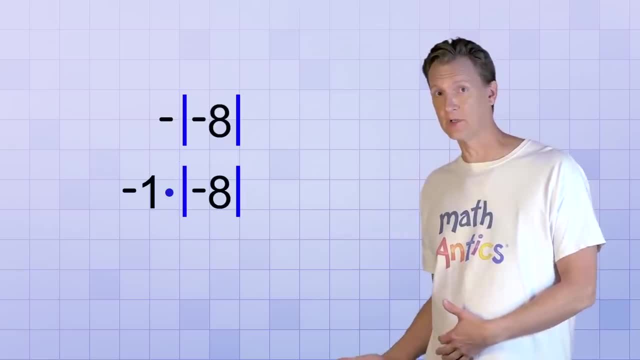 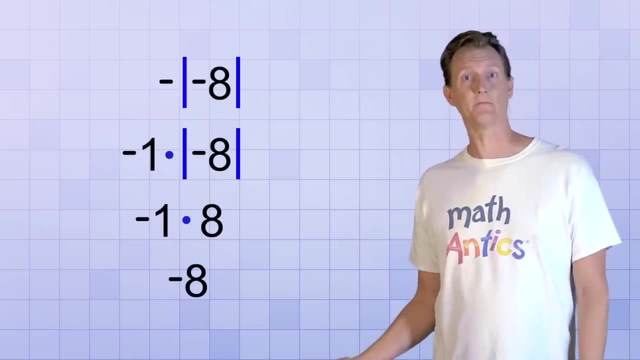 to simplify it, we would first need to do the absolute value. The absolute value of negative 8 is 8.. And then we multiply that by negative 1 and we get the answer negative 8.. That seems pretty simple too, but I want to use this example. 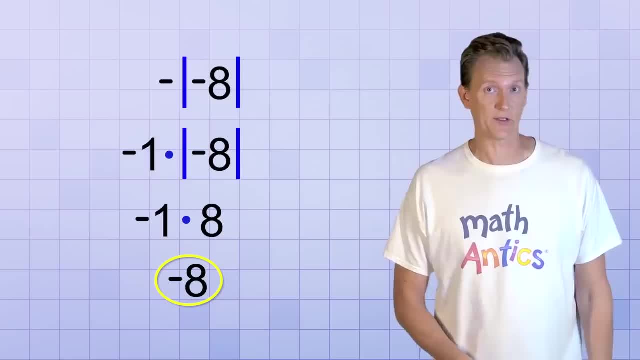 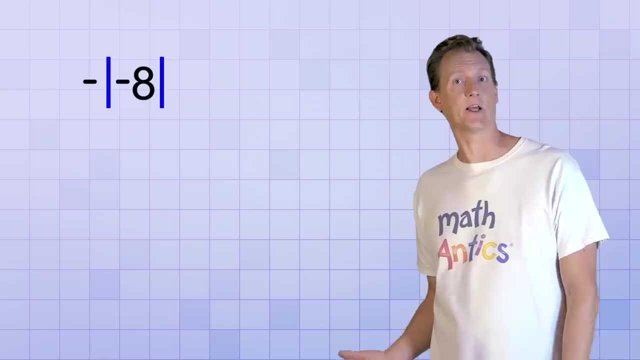 to point out an important difference between parentheses and absolute value signs. It's a difference that can trick you on a test if you're not careful. Let's see the expression we just simplified side-by-side with a similar expression that has parentheses instead of absolute value signs. 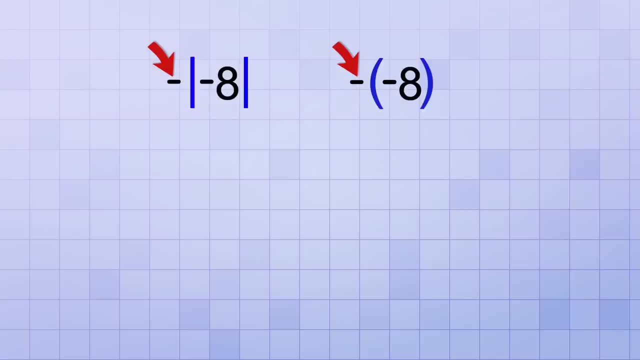 In both of these cases, the negative sign outside the group is telling us to negate the group. That means multiplying it by negative 1.. But there's a very important difference between the two expressions. The order of operations rules tells us to do things that are inside of groups first. right. 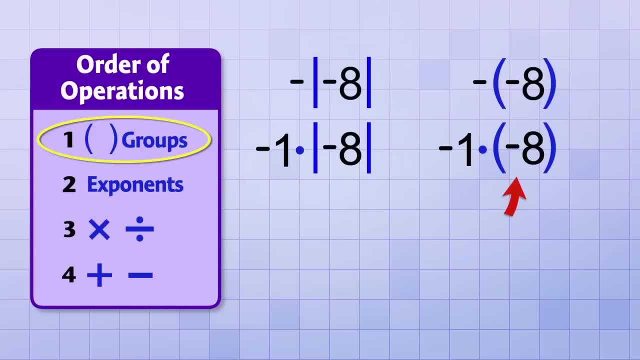 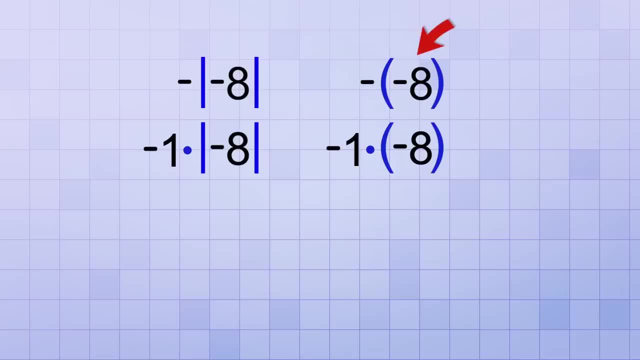 But there's nothing to do inside the parentheses. It's just a negative 8 hanging out inside of them, And the parentheses themselves don't tell us to do anything. So this expression is just asking us to multiply negative 1 times negative 8, which is positive 8.. 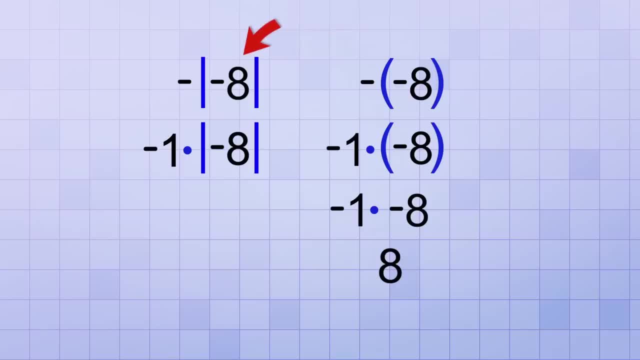 But in the case of the absolute value signs, while they do function like groups, they aren't just for grouping, like the parentheses are. They're also telling us to do something to whatever is inside of them. What are they telling us to do? 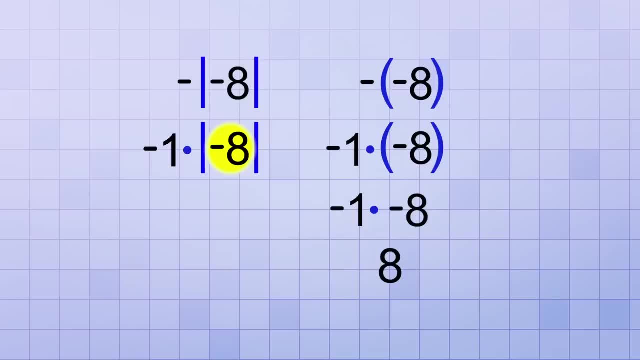 They tell us to use the magnitude of the number inside, which would be positive 8.. So in this expression we multiply negative 1 times positive 8, which simplifies to negative 8.. Do you see how it would be easy to confuse these examples on a test? 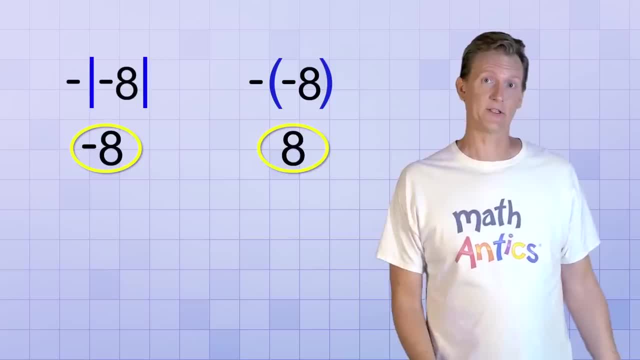 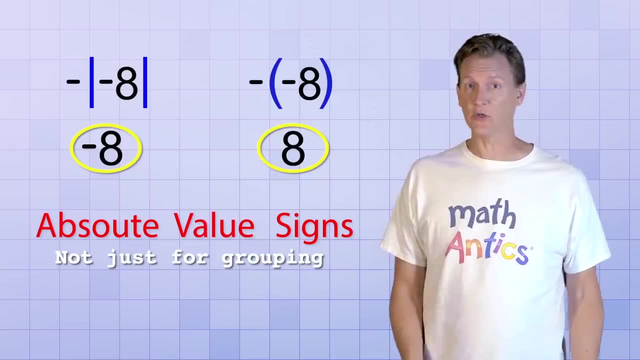 They look similar at first glance but they simplify to different answers. The key is to always remember that absolute value signs are not just there to group things. They're also asking you to find the absolute value of whatever number or expression is inside the group. 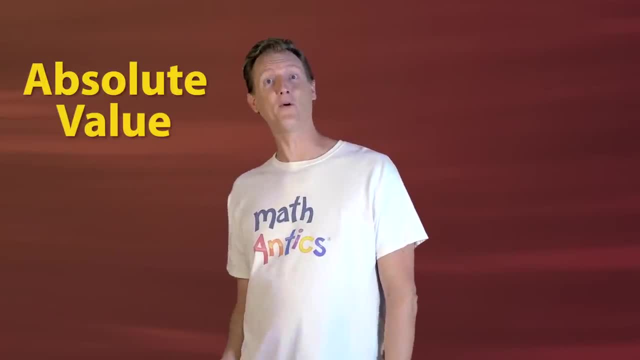 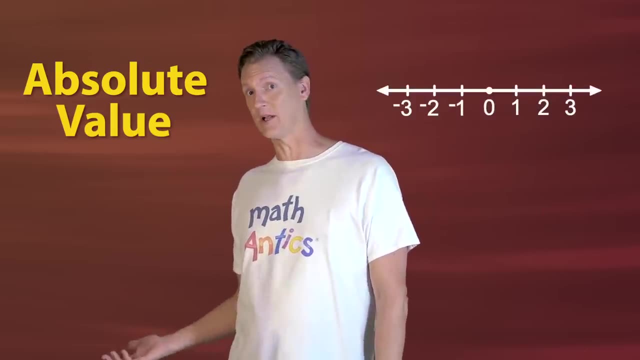 Alright, as you can see, absolute value is a lot more than just a way to turn negative numbers into positive ones, Although that's basically what it does when you're just dealing with numbers on the number line- But it has lots of other applications in math too.